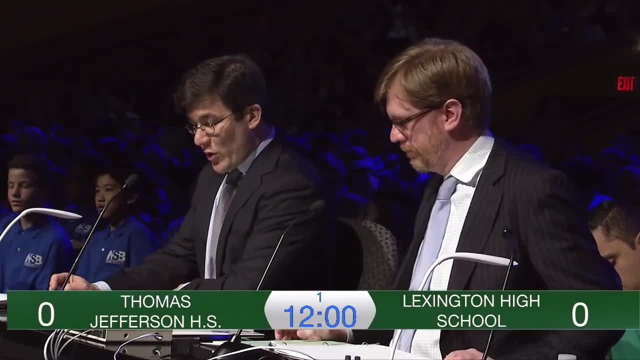 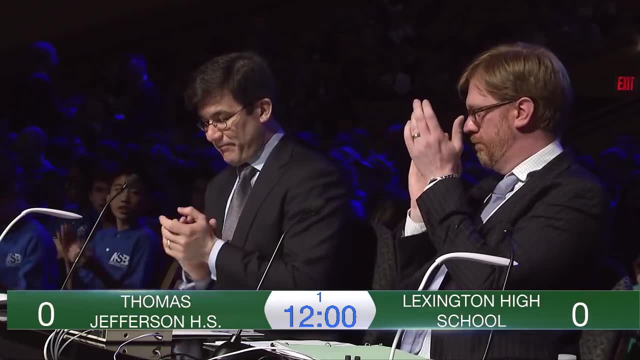 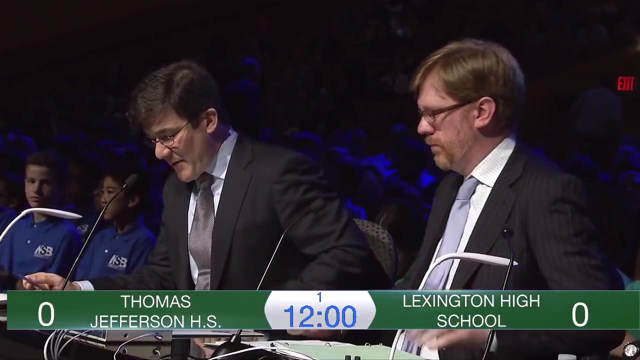 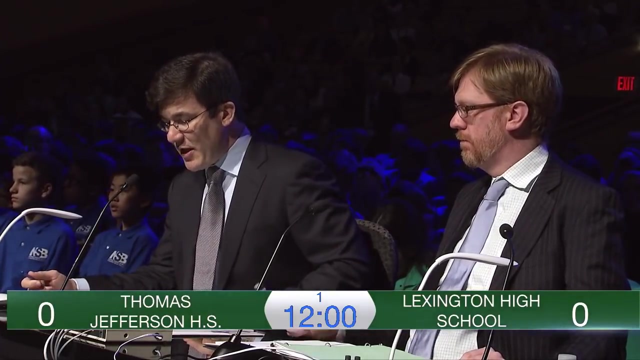 Welcome to the High School Finals of the 2017 Department of Energy National Science Bowl Competition. At this time, I'd like to welcome our two finalists to the stage: Team A hailing from Alexandria, Virginia, coming in with one loss from double elimination. 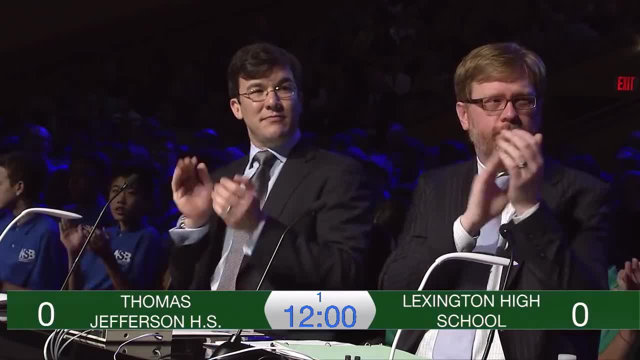 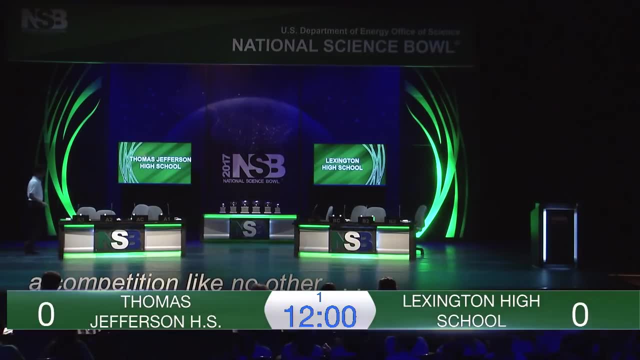 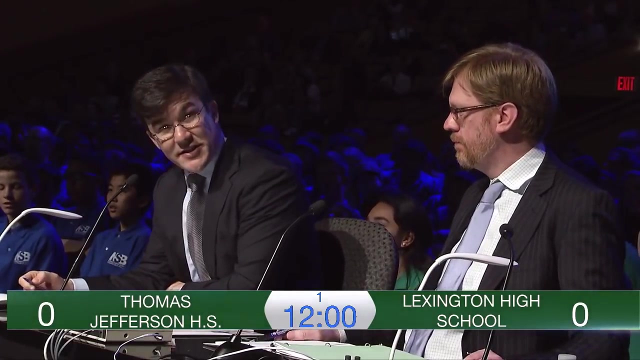 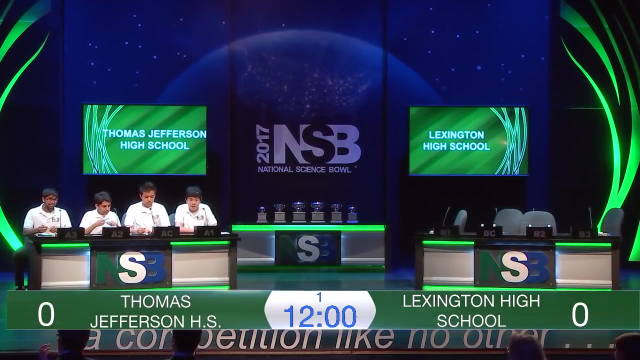 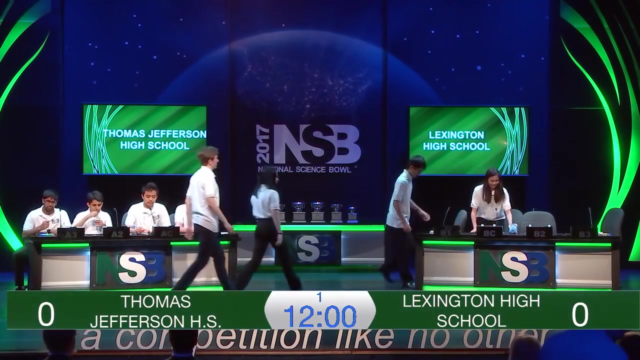 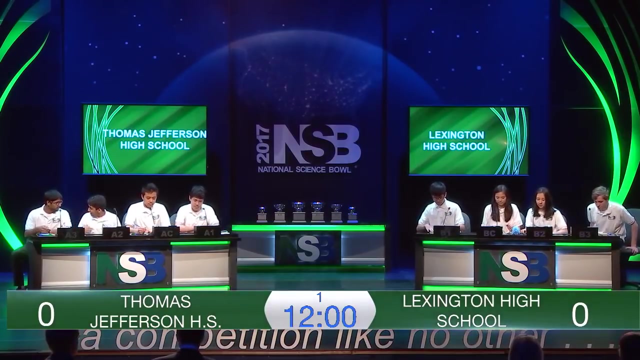 Thomas Jefferson High School for Science and Technology And Team B, hailing from Lexington, Massachusetts, coming in with no losses. Lexington High School. Okay, at this time we'd like to test the buzzers and have the contestants introduce themselves to us. 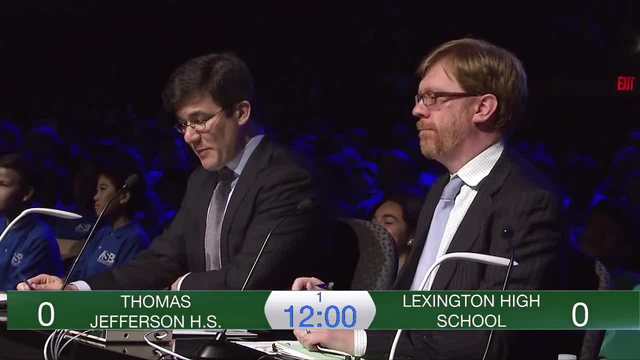 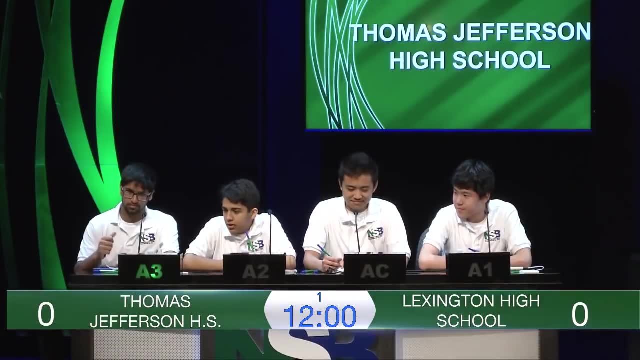 Please buzz in wait to be verbally recognized by Phalem. Tell us your name, your year in school and what career you'd like to pursue after your education is completed. A3.. Hi, I'm Neeraj, Grade 12,, and I'd like to pursue biochemistry. 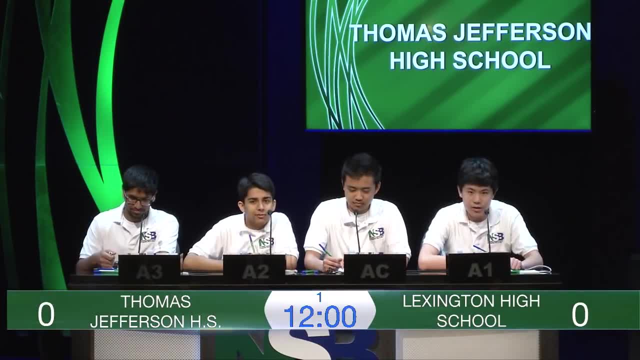 A2.. Hi, I'm Aditya. I'm a sophomore and I'm interested in artificial intelligence. A-Captain. Hi, I'm Franklin. I'm a junior. I always knew I wanted to do research, but I didn't know where. 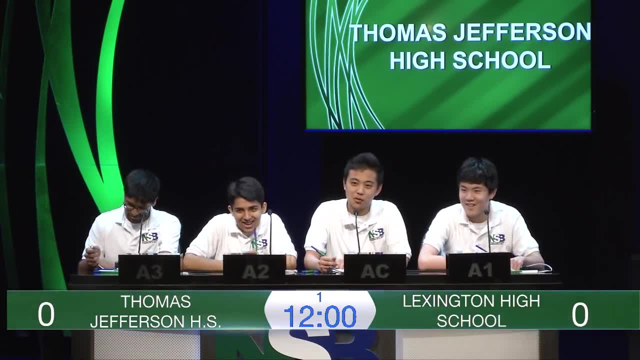 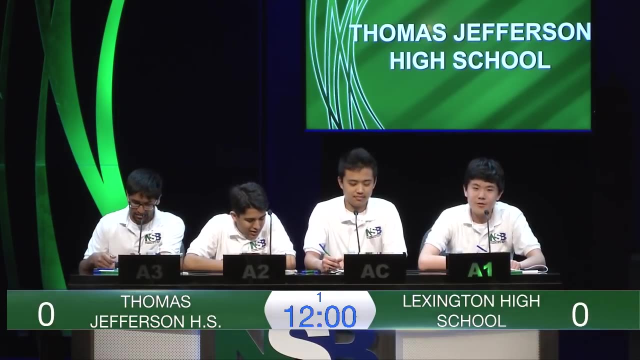 Now I know where, after listening to all the questions, this weekend I'd like to go to Lawrence Livermore National Lab. That's a great answer. A1.. Hi, I'm Charles Wong. I'm a junior. I guess I'd go into particle physics, study goldstone bosons, that sort of stuff. 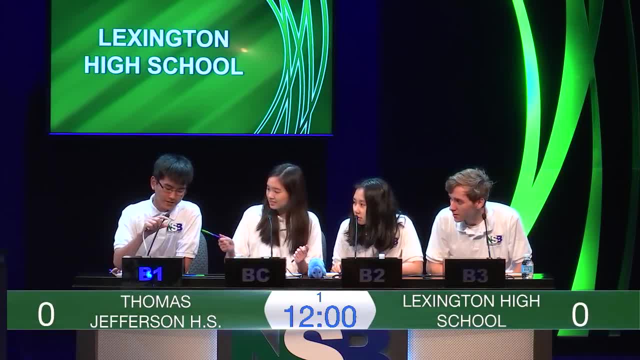 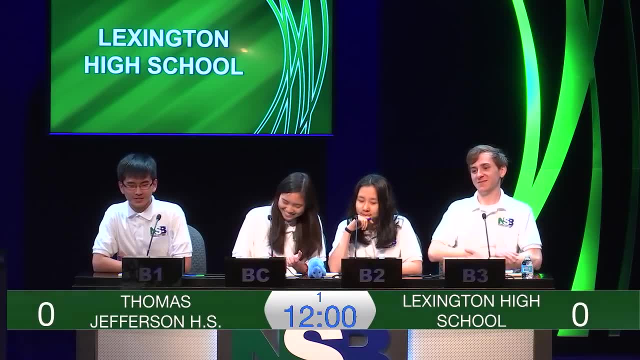 B1. I'm Joshua. Sorry, Joshua, please speak into the microphone. Joshua, I'm a junior and I want to become Ben Choi, the chemist's boy. B2. B-Captain- Hi, I'm Katherine. 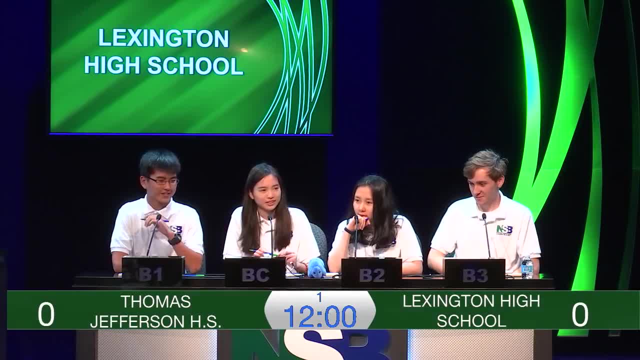 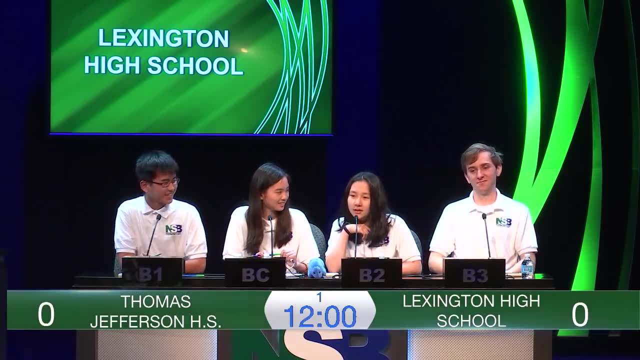 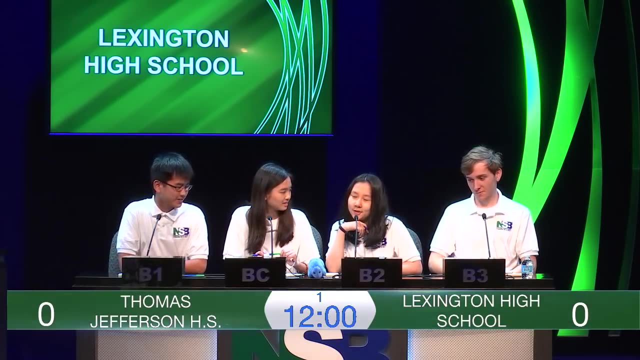 I'm a senior at LHS and I want to be Ben Choi, the physician-scientist boy B2.. Hi, I'm Anka, I'm a freshman at LHS and I want to be Ben Choi, the Meisner-Oschenfeld effect boy. 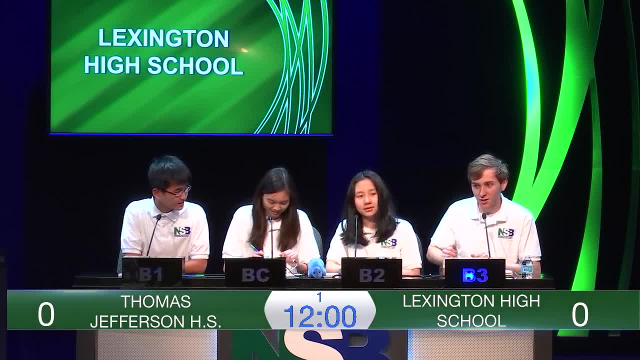 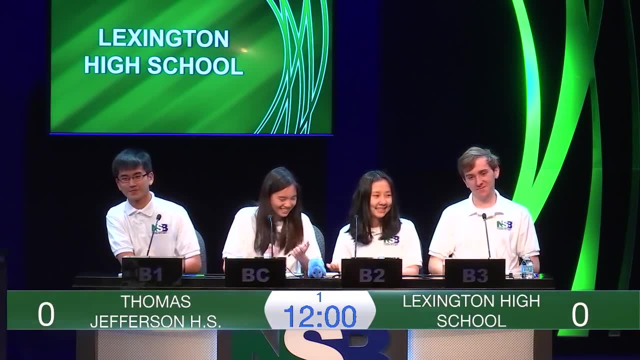 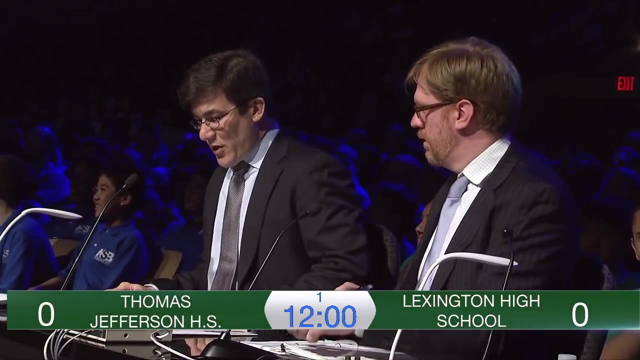 B3.. Hi, I'm Derek Hoffman, a junior at LHS, and I want to be Ben Choi, the particle physics boy. All right, thank you very much. Okay, so, as I said, Thomas Jefferson High School currently is coming in with one loss. 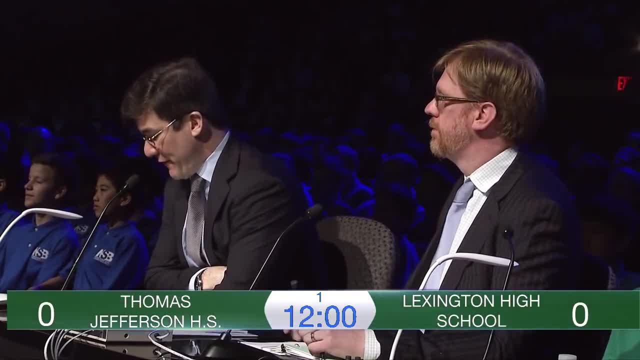 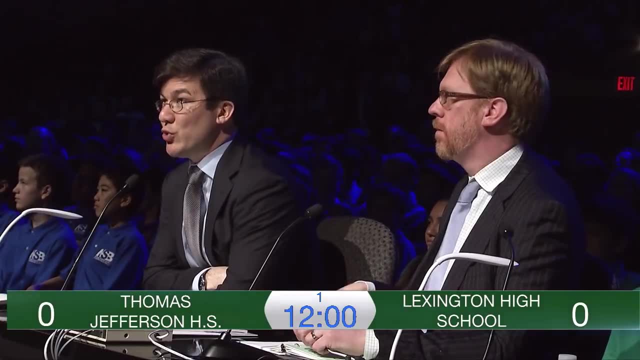 Lexington High School coming in with no losses. So that means that if Lexington wins round eight, they will be our champions and Thomas Jefferson will be our second-place team. If Thomas Jefferson wins round eight, then we'll go to round number nine. 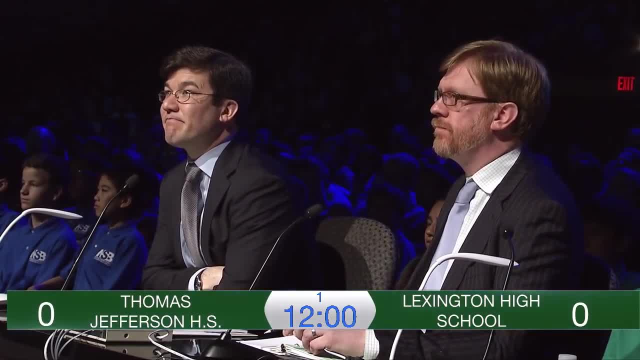 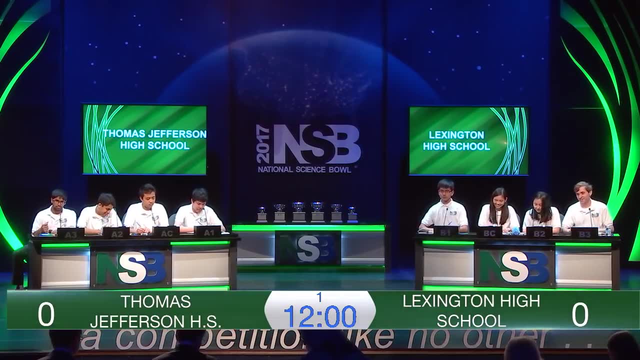 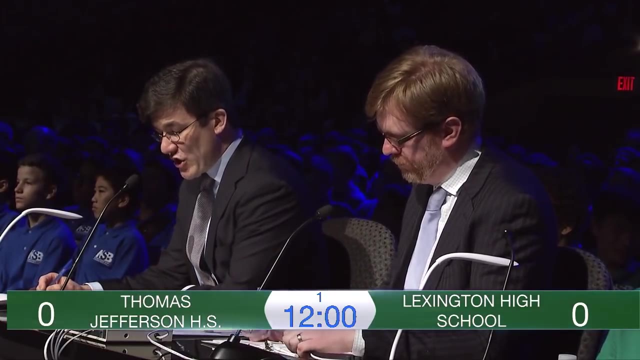 Do we have any questions before we begin? Are both teams ready? Team A: Yes, Team B: Yeah. Best of luck. Without further ado, let's begin. This is High School Dublimination, round number eight. First question: toss-up: biology. short answer. 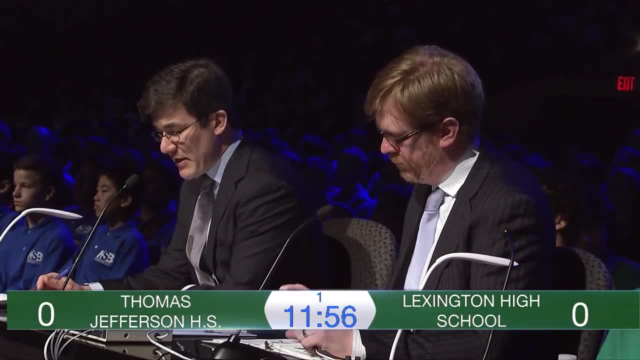 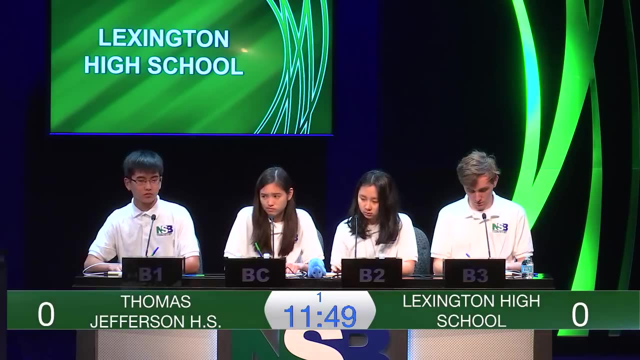 The cytosol of cells is thought of as a reducing environment, mainly due to the presence of wet sulfur-containing molecules. B, Captain Sistine, I'm sorry that's incorrect. A1. Sulfate- Sorry, that's actually glutathione. 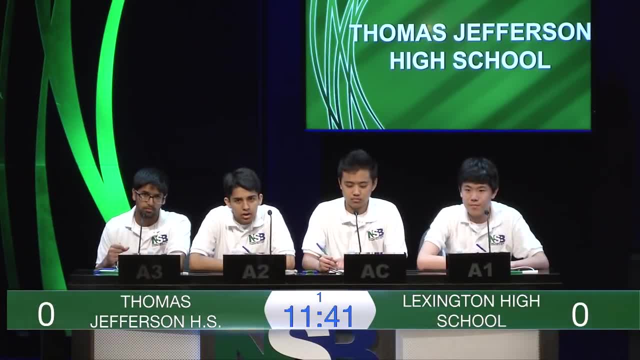 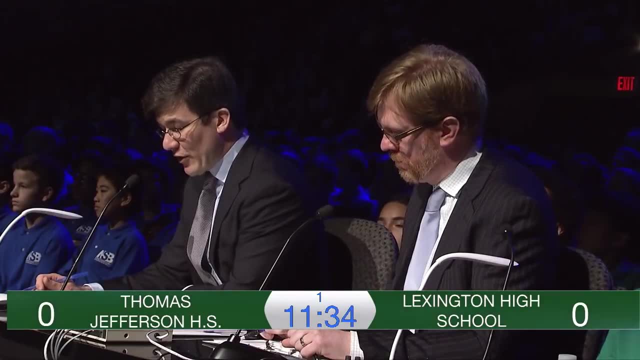 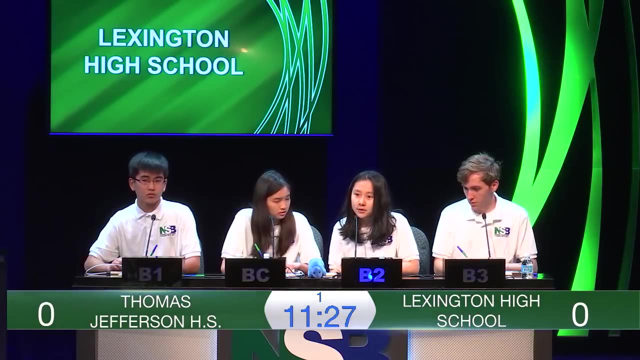 Toss-up number two is in physics. short answer: After being exposed to an external magnetic field, a ferromagnet does not relax to zero magnetization when the field is removed. Interrupt B2.. Hysteresis Is correct. 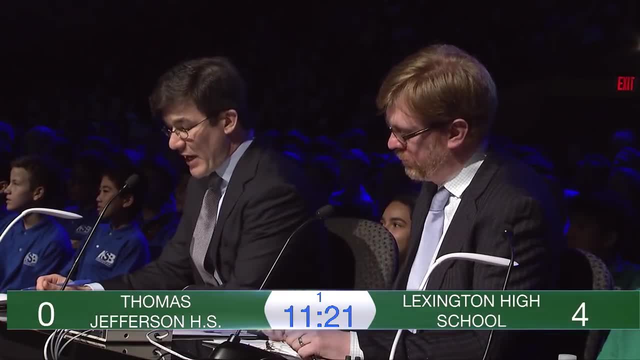 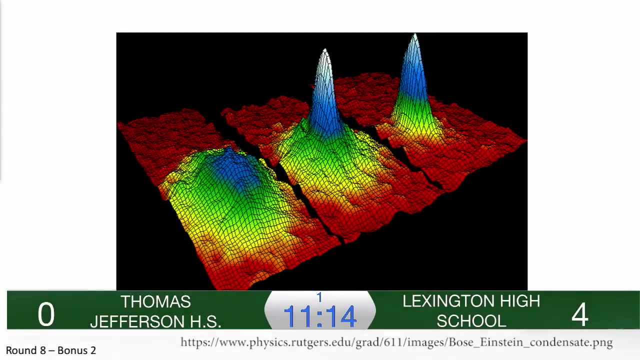 Your bonus question is visual in physics and short answer: Depicted is the velocity distribution. We don't see anything. Sorry, stop the clock please. Please tell me when the display is showing. Oh, they're not showing. You guys are good. 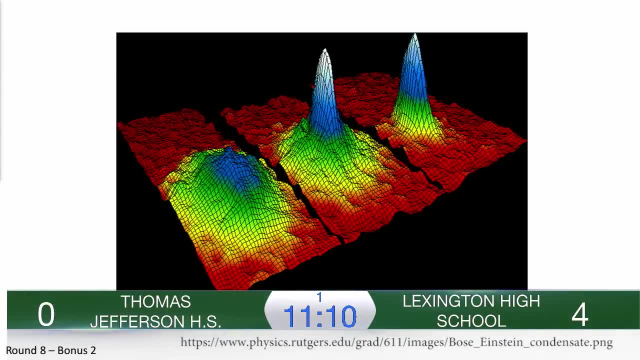 Yeah, Okay, physics- short answer: Depicted is the velocity distribution of an ultra-cold gas as it undergoes a phase transition. Answer the following two questions about the image. One: what state of matter has been formed? Two: indicate all of the following three neutral atoms that could compose this state. 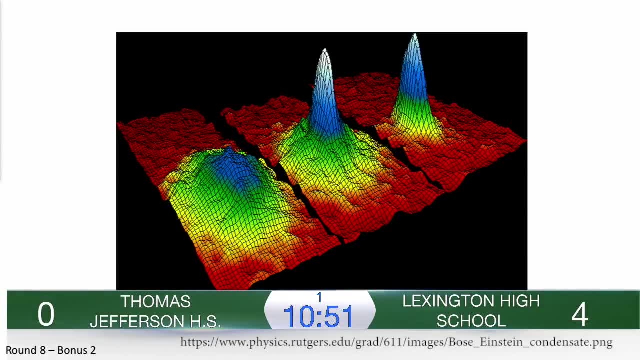 A, deuterium B, helium-4, C, sodium-23.. Okay, So it's boson and condensate and you want bosons, So helium-4, deuterium is. Is deuterium a boson? 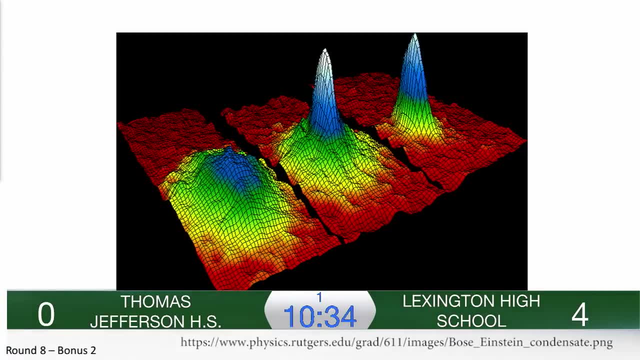 I think it is, I don't know, One proton, one neutron. So let's say One One. One is Bose-Einstein condensate, Two is A and B, Or Yeah, it's A and B, right. 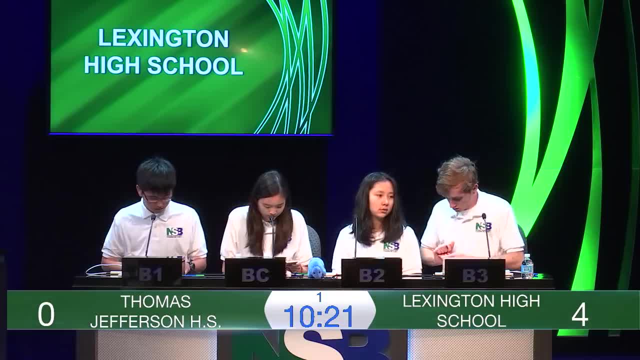 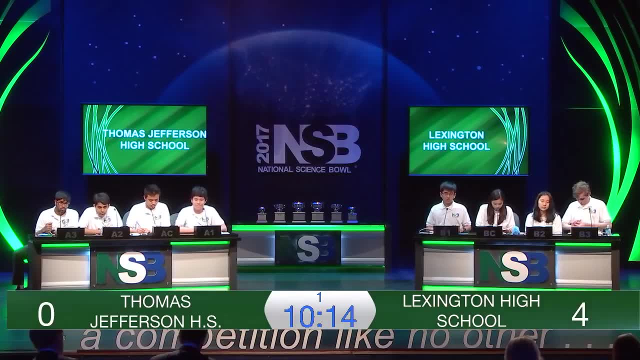 Okay, yeah, Okay. One is Bose-Einstein condensate. Two is deuterium and helium-4.. Sorry, it is a Bose-Einstein condensate, but it is helium-4 and sodium-23.. Toss-up. three is an energy multiple choice. Department of Energy, scientists at Los Alamos National Lab changed three amino acids on the enzyme carbonic anhydrase to enhance its thermal stability. Which of the following changes would be most likely to increase stability but would not interfere with its catalytic cycle? 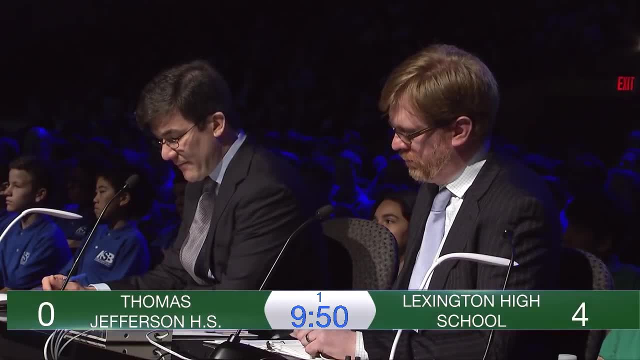 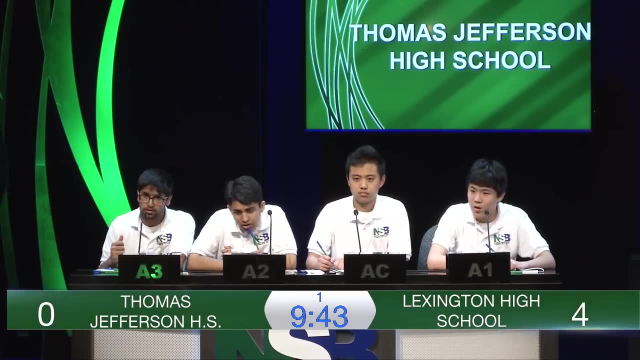 W. changing three aspartate residues at the active site to valine. X. changing three outward-facing hydrophobic residues to aspartate Interrupt A3.. X Is correct. Your bonus question is visual in energy and it is short answer. 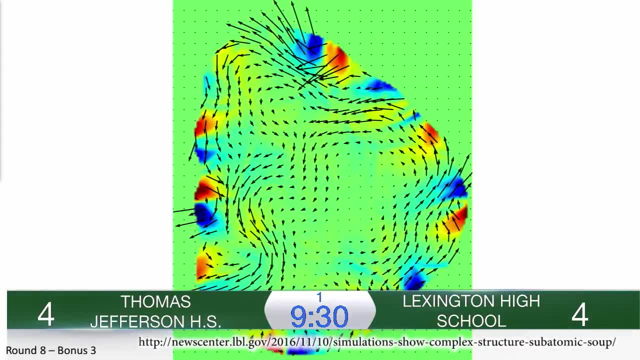 The image shows a simulation of the flow pattern of the enzyme carbonic acid. The image shows a simulation of the flow pattern of a fluid created in the relativistic heavy ion collider at Brookhaven National Lab. Answer the following two questions about the image. 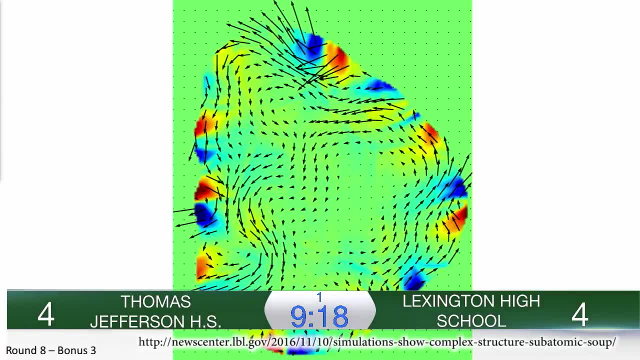 One: what is the common name of this fluid that was first discovered in the RIC in 2005?? Two: identify all of the following three particles that, when collided in the RIC, can produce this fluid: One: electrons. Two: gold nuclei. 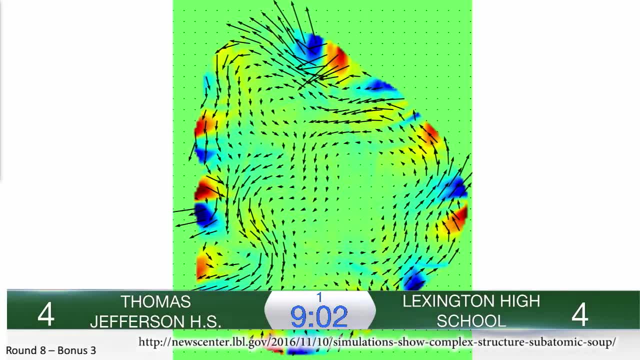 Three protons. Okay, so it's ortho and plasma. I think this is a good question. It would be two only. Why not three? Because like there's not enough stuff in there to be a good question. Okay, so quark gluon, plasma and two only. 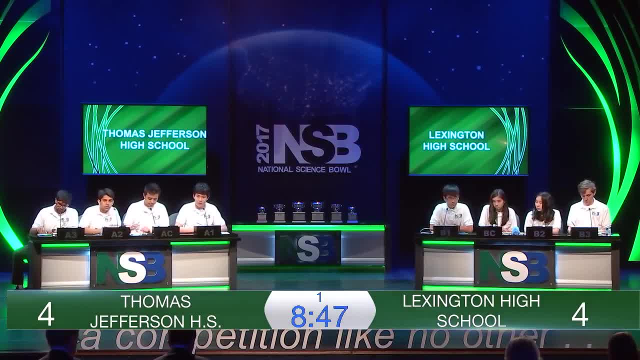 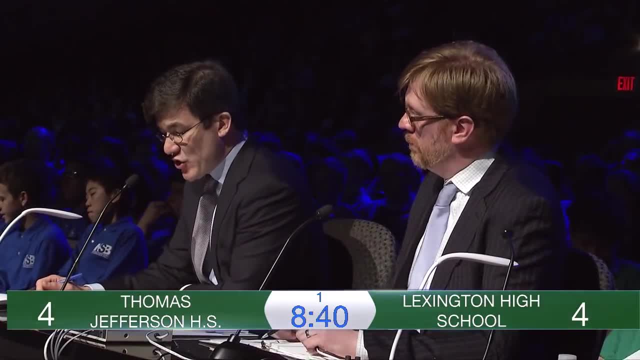 Okay, quark gluon plasma and two. only It is a quark gluon plasma and unfortunately it is two and three. Pass up four: earth and space. short answer. A white dwarf star resists gravitational collapse due to the degeneracy of what interrupt. 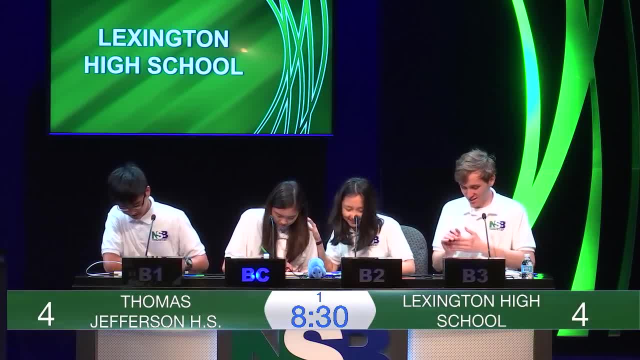 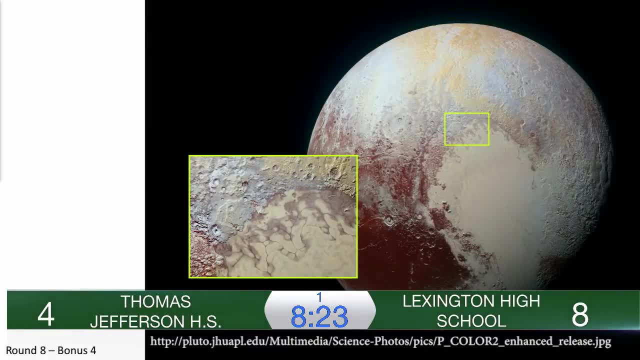 B captain Electrons Is correct, Nice. Your bonus question is: visual in earth and space. short answer: On the screen is an image of Pluto compiled by NASA's New Horizons team. Identify all. It's not Okay. now we're good. 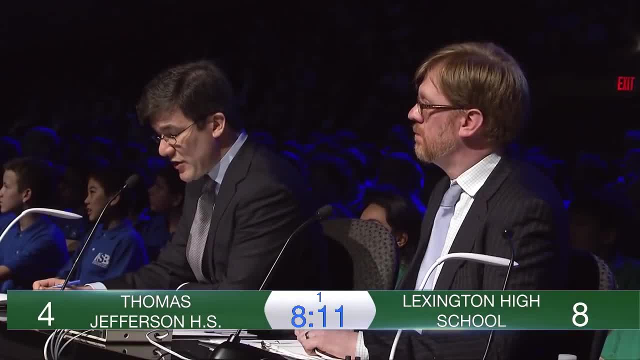 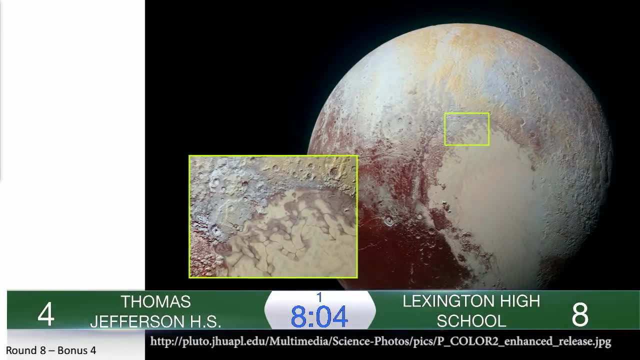 Sorry, I'll start over Earth and space. short answer. On the screen is an image of Pluto compiled by NASA's New Horizons team. Identify all of the following statements that are true of the unit of high albedo surface material known as: 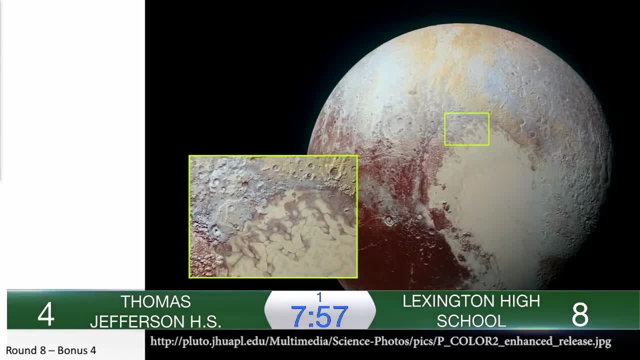 Ecos headquarters. isotropic planum One: it is composed primarily of water ice. Two: it is thought to be slowly convecting. Three: it unlapsed geologically older surrounding terrain. Three is probably right: Water ice. I don't think it would be conveiamente. 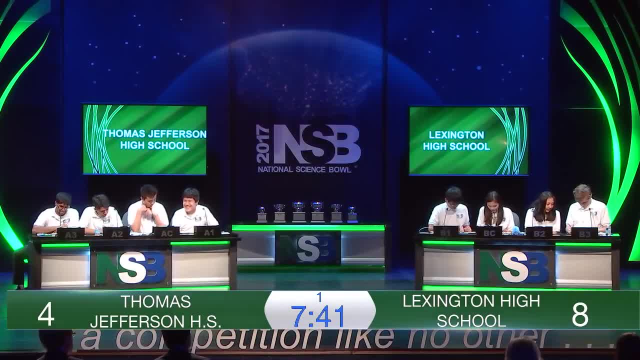 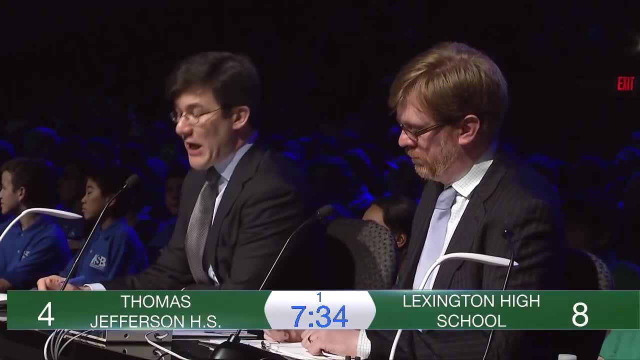 That means it is liquid or gas, right? Yeah, that seems sketchy. so I think it is one and three. Okay, one and three. Sorry, it was actually two and three. Toss it number five for both teams and chemistry. short answer. 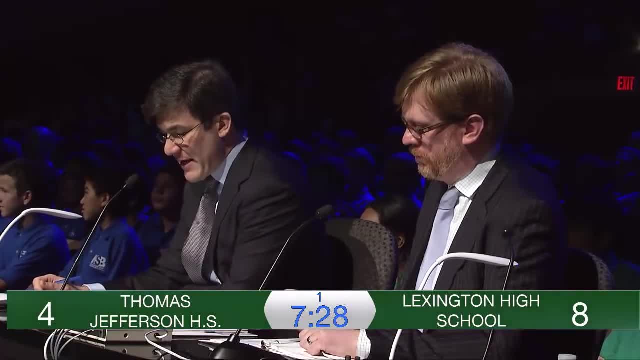 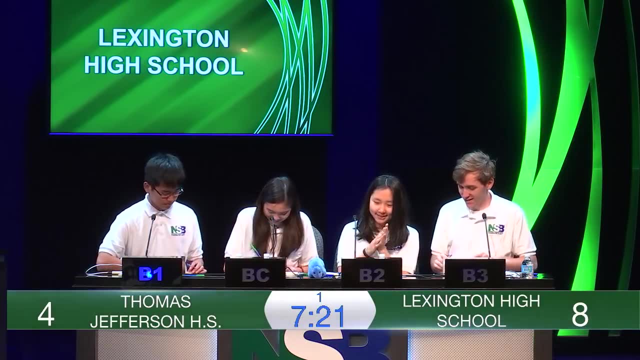 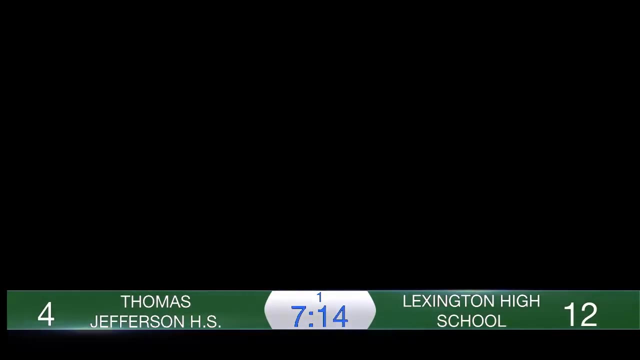 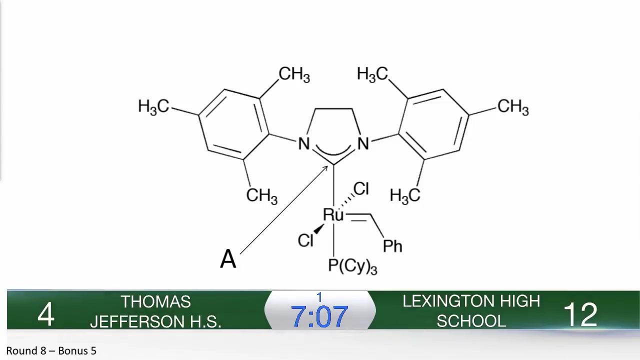 In organic chemistry, saturated rings, with what number of atoms have the largest relative formation rates in ring interrupt? E1.. 5. Is correct, Nice. Your bonus question is visual in chemistry. short answer Shown on the image- is a ruthenium-based catalyst. 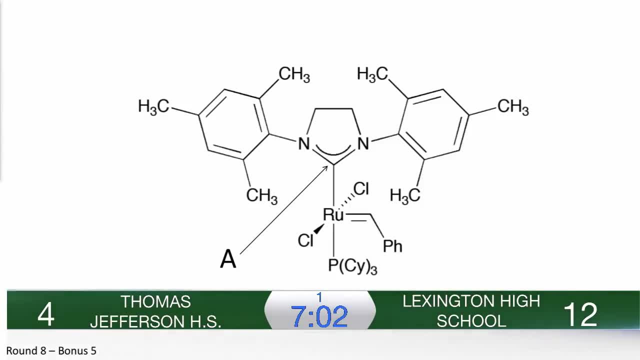 used for the olefin metathesis reaction, which was developed by Robert Grubbs as part of the work that won him the Nobel Prize in Chemistry in 2005,, along with Chauvin and Schrock. Answer the following two questions regarding the image. 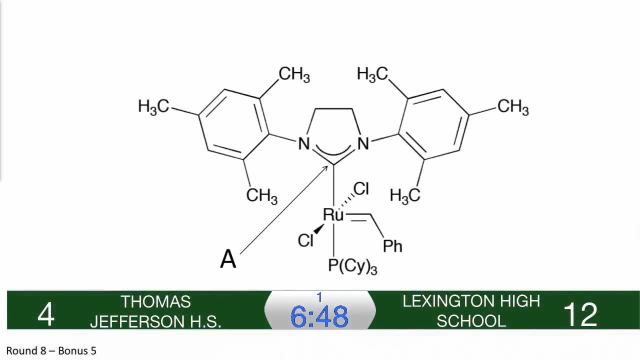 One: what is the oxidation state of the central ruthenium atom? Two, what functional group present on the unusual ligand labeled A consists of a hypovalent carbon atom donating its lone pair to the metal. Okay, two is a carbene and I think one is two. 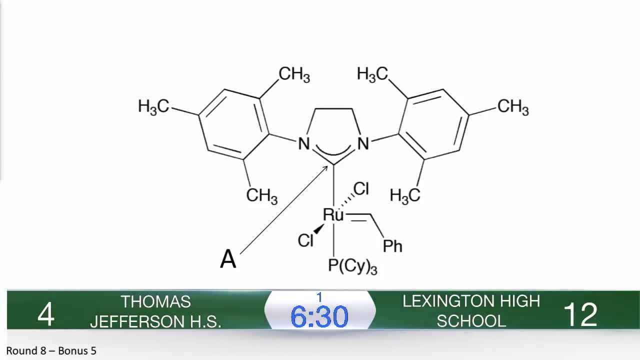 Let's see, We have some time. Should I say two plus Yeah, Station here this thing: Two plus and carbene. Okay, one is two plus two is carbene. Sorry, one is plus four, but two is carbene. 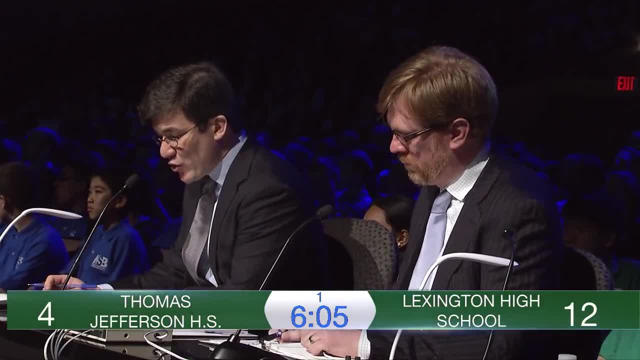 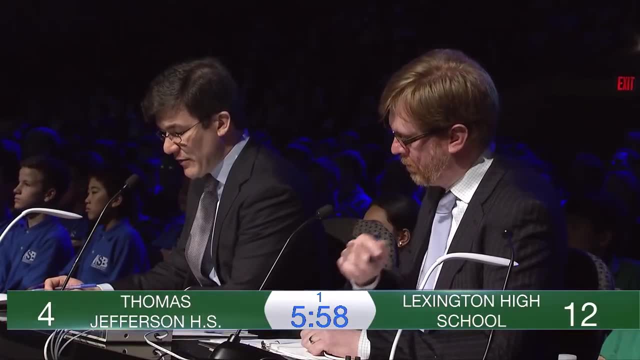 Toss-up. six is in math. short answer: Find the quadratic polynomial with integer coordinates and smallest positive leading coefficient that has the same sum and product of zeros as 3x to the 7th minus 5x to the 4th plus 6x plus 2.. 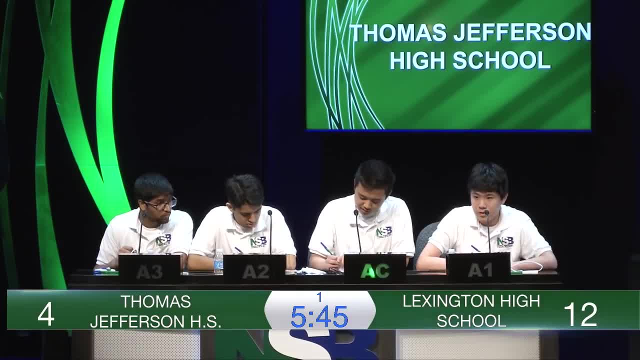 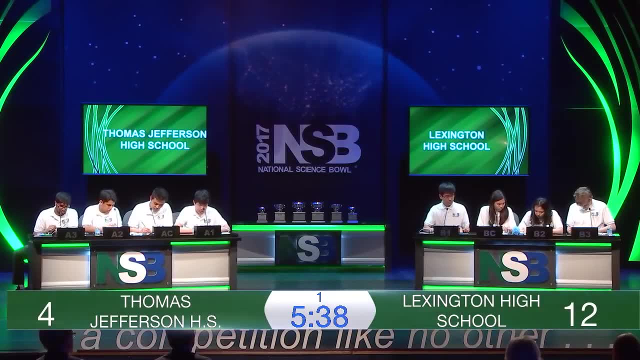 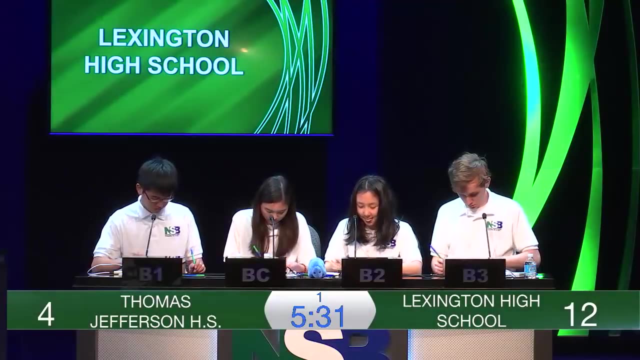 A captain: 3x squared minus 5x plus 2.. I'm sorry that's incorrect- B2.. 9x squared minus 15x plus 4.. Sorry, it's incorrect. It's 3x squared minus 2.. 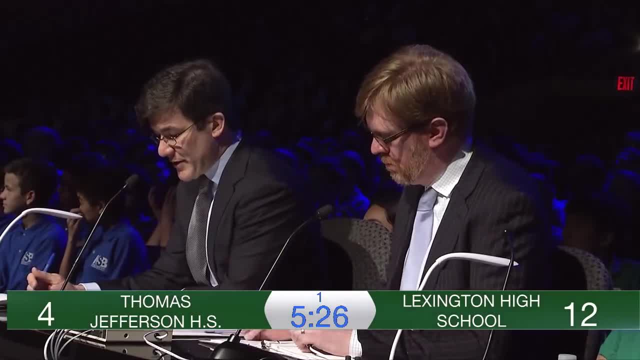 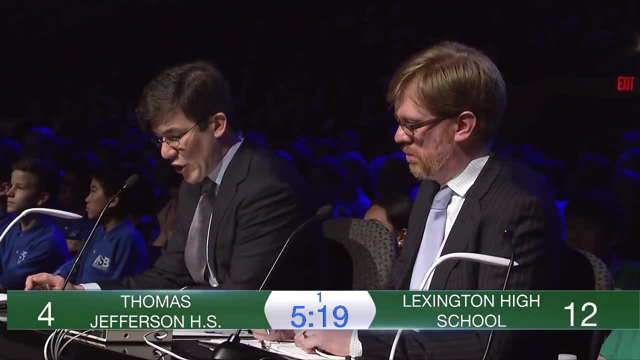 It's okay. It's okay Toss-up seven physics multiple choice. Which of the following is not a region of a bipolar junction: transistor W, base X, emitter Y, gate Z, collect Interrupt B3.. 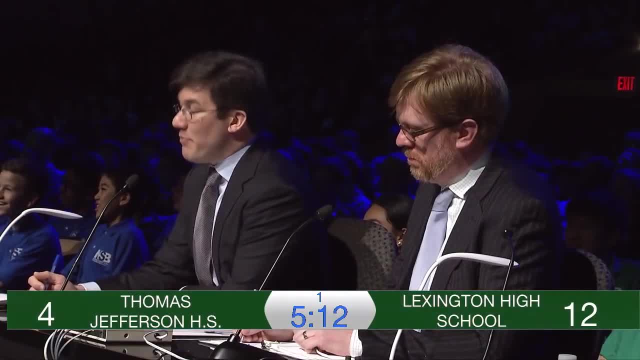 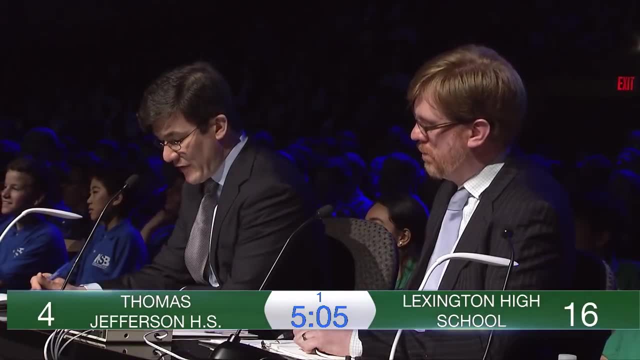 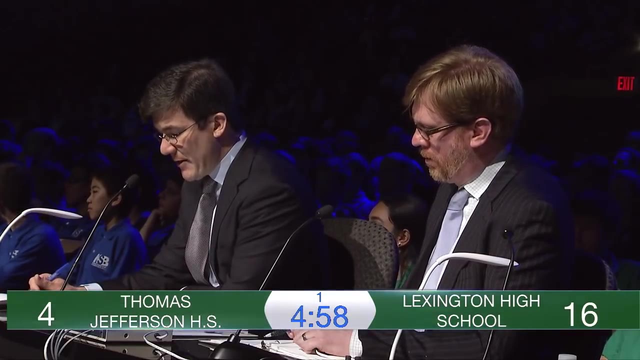 Y Is correct. Sorry, I blanked on that. Bonus physics short answer. In Cartesian coordinates the electric potential in a region is described by the function 1 minus 1.. Y, z squared. Calculate the electric field at the point negative: 3,, 3,, 5.. 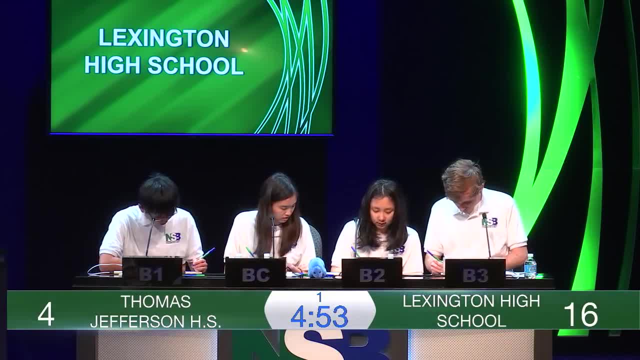 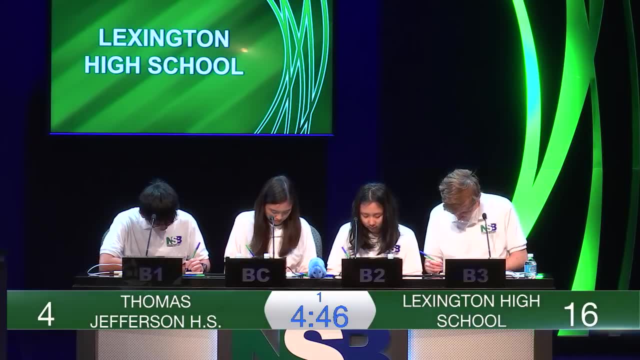 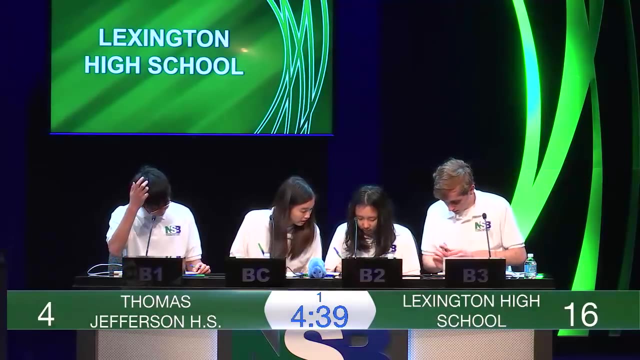 So we have to do the derivative. Yeah, so it's. So that's minus z squared, and then minus y, minus 2yz. So that should be minus 25, minus 2yz, Minus 55.. Minus 55.. 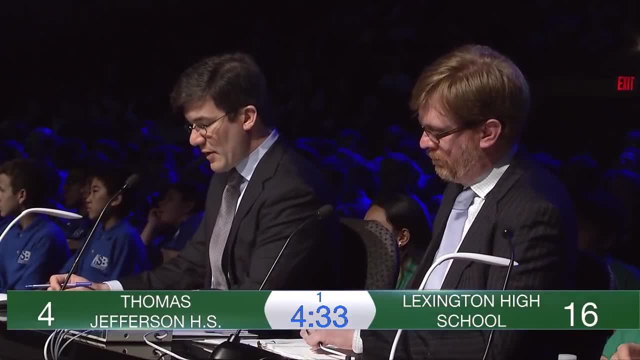 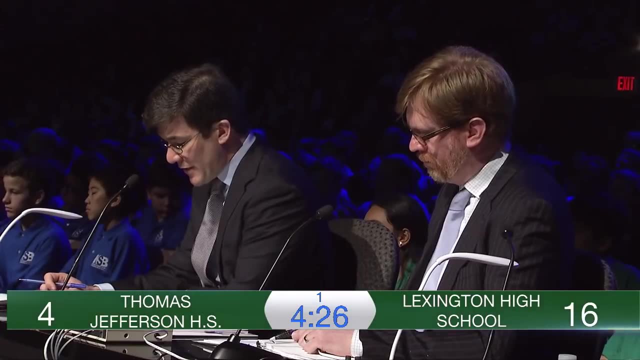 Sorry, it's 25j plus 30k. Okay, Toss-up eight. chemistry. short answer: Consider the reaction of the organometallic reagent phenyl lithium with formaldehyde at minus 78 degrees Celsius. What functional group is formed in this reaction? 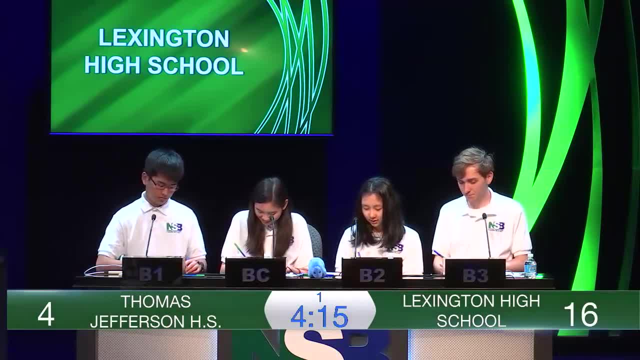 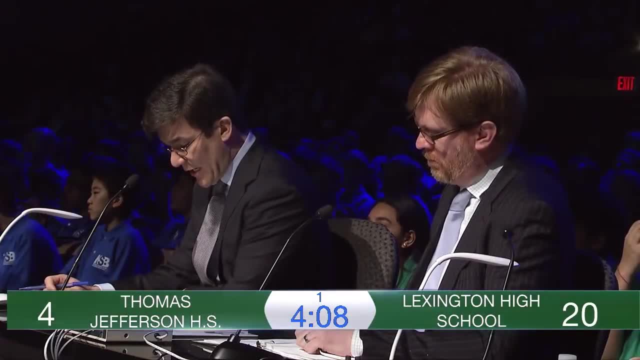 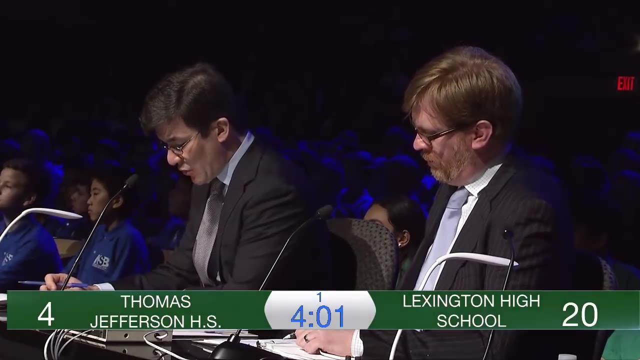 B1. Alcohol Is correct. Your bonus in chemistry is short answer. Rank the following three hydrogen atoms in increasing order of pKa: One hydrogen alpha to two ester carbonyl groups. Two hydrogen alpha to two ketone carbonyl groups. 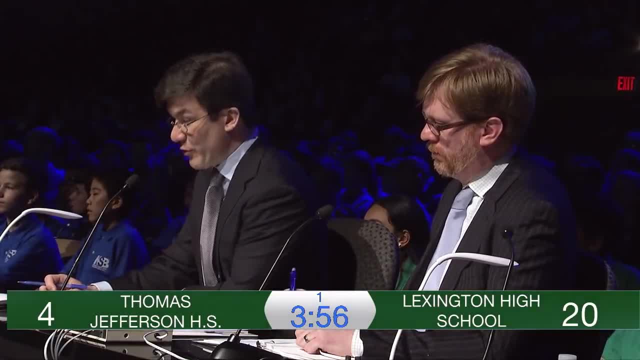 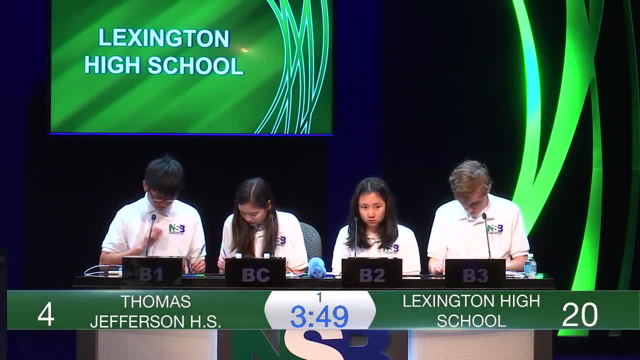 Three hydrogen alpha to single ketone carbonyl group. Okay, so that would be 2, 3, 1.. 2, 3, 1?? Uh-huh, You have some time to check it if you need to. 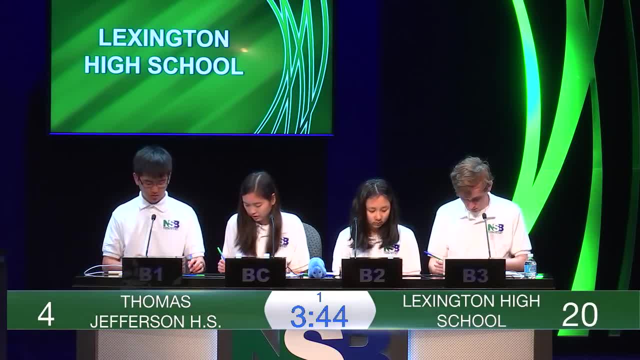 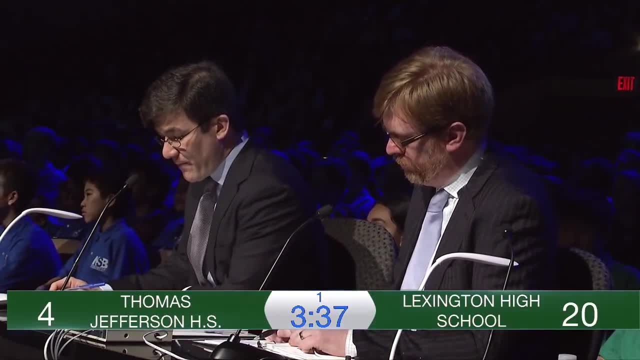 I think we've seen some of this. Yeah, 2, 3, 1.. 2, 3, 1.. Sorry, it was 2, 1, 3.. Toss-up nine is in biology. short answer. 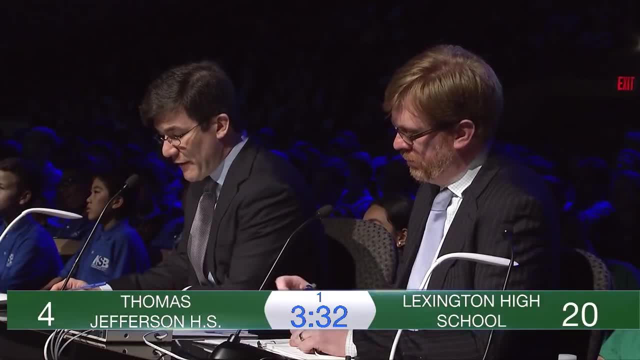 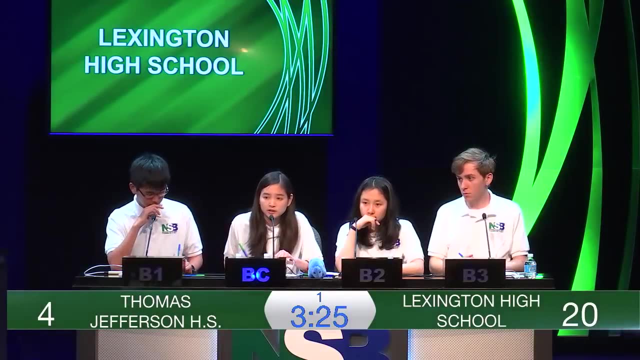 Vasopressin stimulates the action of phospholipase lipase C on phosphatidyl inositol 4, 5-bisphosphate releasing IP3 and what other interrupt B captain Diatylglycerol. 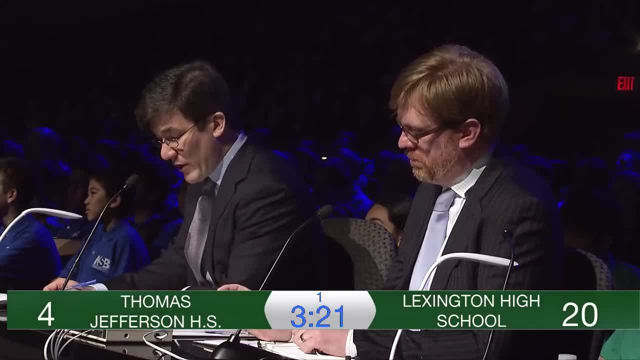 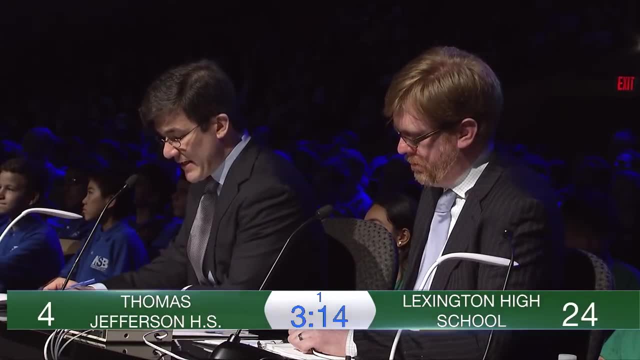 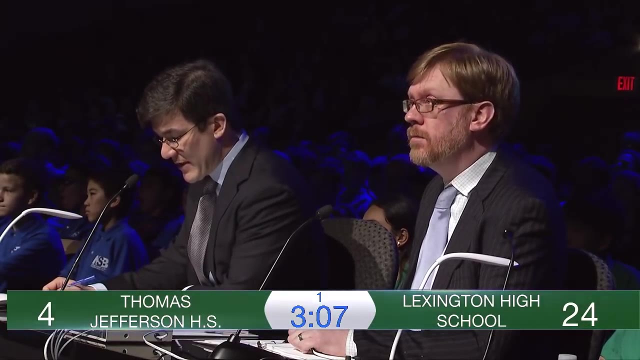 Is correct. Your bonus in biology is short answer. Identify all of the following three statements that are true regarding apoptosis. One: cytochrome C released from mitochondria causes apoptosis. That's true. Two: cytochrome C has proteolytic function outside of the mitochondria. 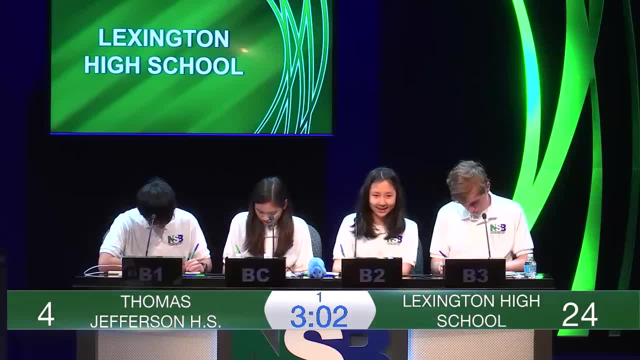 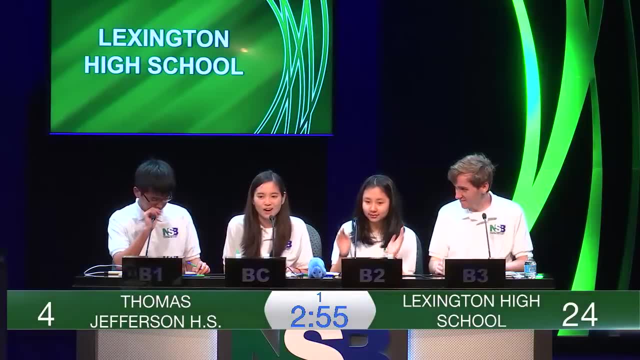 Don't think so. Three caspase: 9.. Is a protease Caspase? Yeah, Dude, they got that wrong. Okay, I think it's 1, 3.. Yeah, Whatever, 1, 3.. 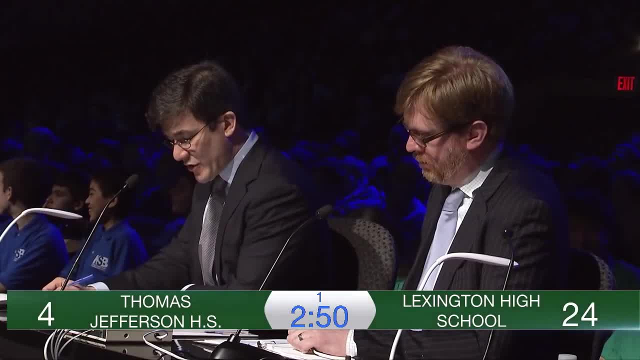 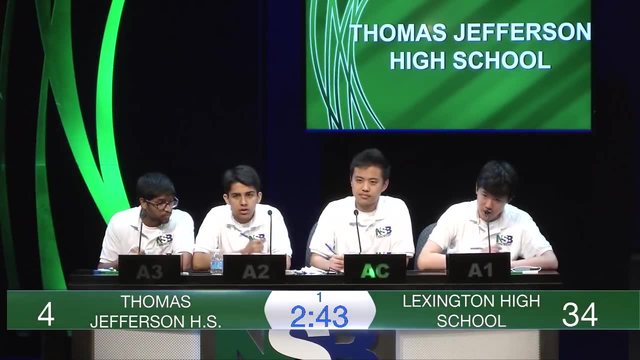 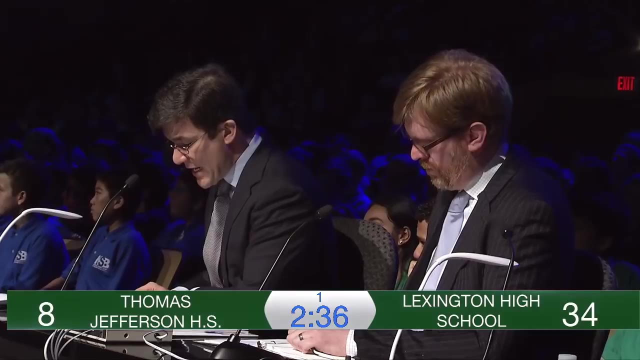 Is correct. Nice Toss-up 10, math short answer. How many edges are in a complete graph with 12 vertices? A captain 66.. Is correct? Your bonus question in math is short answer. Each of the integers from 1 through 10,000 are written on 10,000 cards. 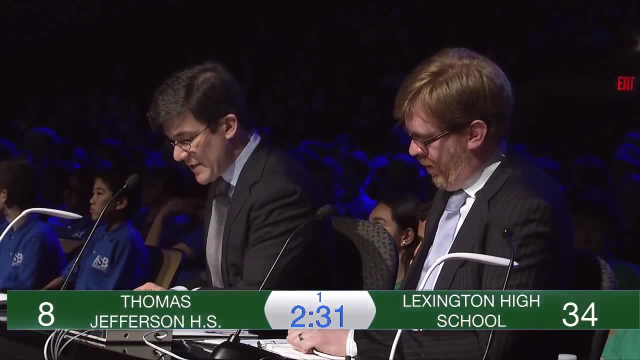 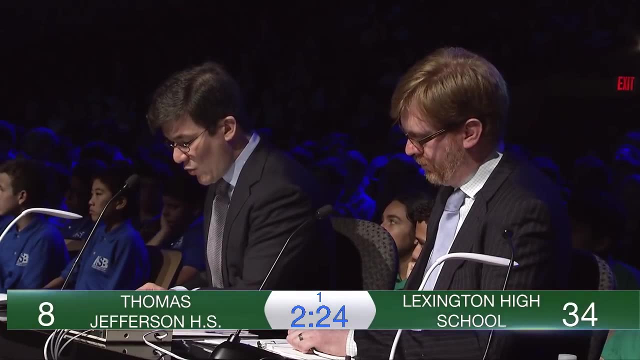 Ok, One on each card, which are then stacked in order, with one on the bottom and 10,000 on the top. The cards are then dealt: two cards from the top of the stack, then one card from the bottom, and then repeating this process to deal all the cards. 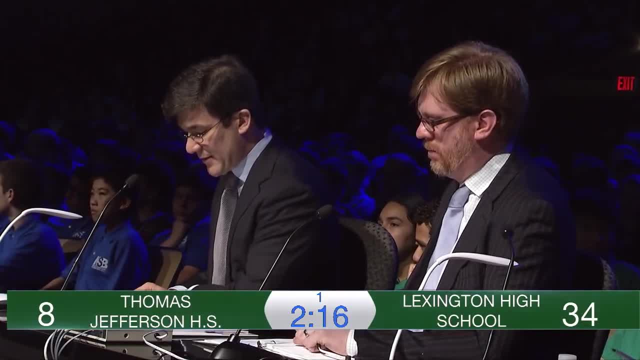 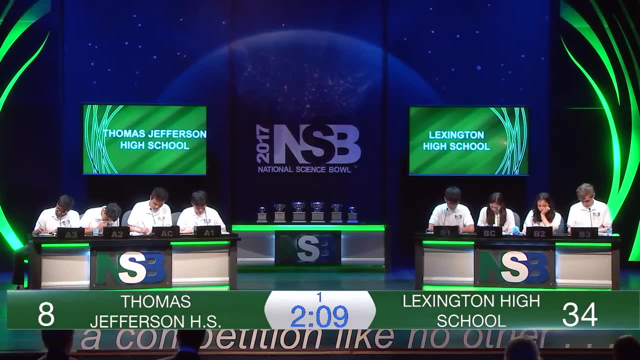 What is the number on the 2017 card dealt? 7,, 9,, 7,, 7.. Sorry, It's 8,, 6, 5, 6.. Toss-up: 11, energy short answer. 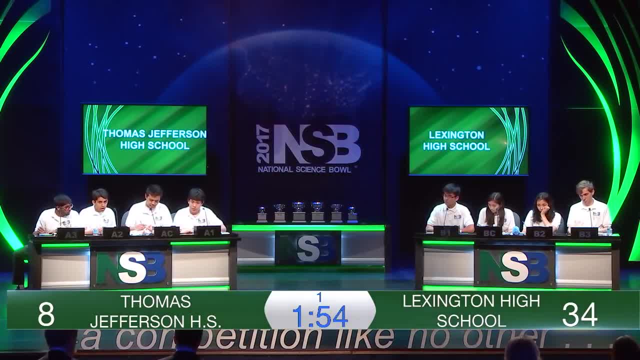 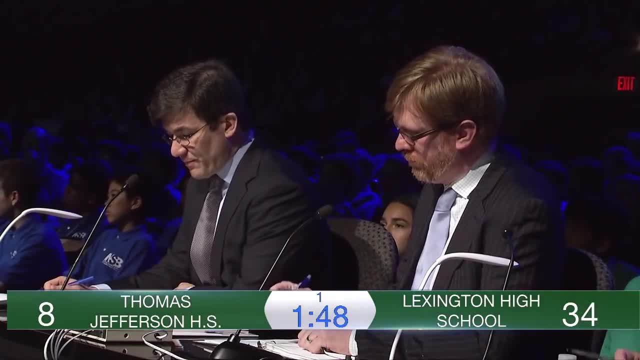 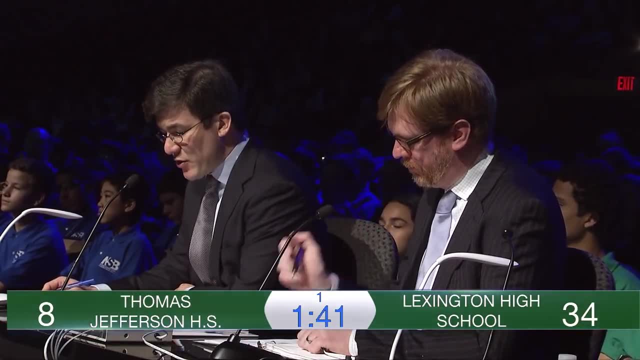 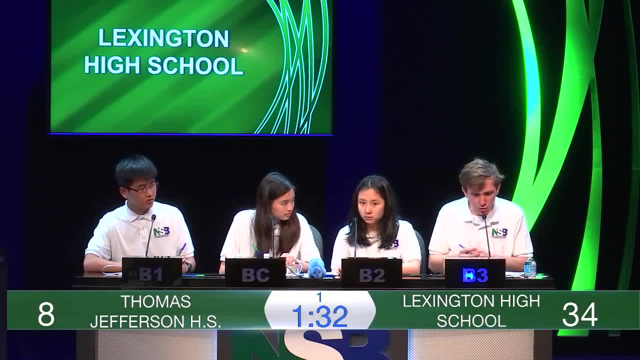 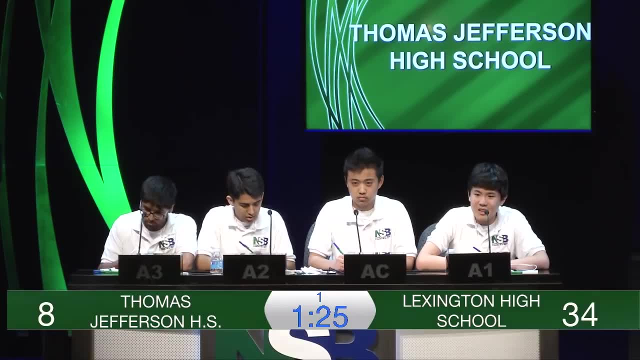 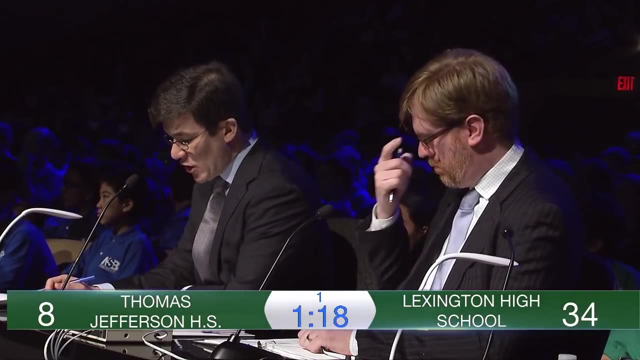 b3 penta corpse. i'm sorry that's incorrect a1 mesons. sorry, it's actually the b mesons. toss up 12: earth and space multiple choice. in the late 1800s, lord kelvin estimated the age of the earth to be approximately 100 million years. by calculating how long it would take a planet of earth's size to cool from its temperature of formation. kelvin's estimation was under the true value of 4.5 billion years because he neglected what source of heat interrupt a1 radioactivity. sorry, it's incorrect. i'll repeat for team b: 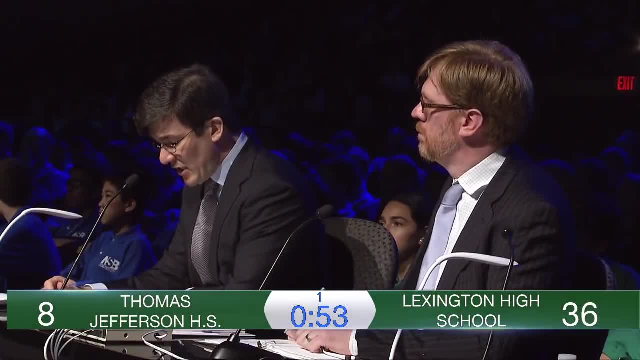 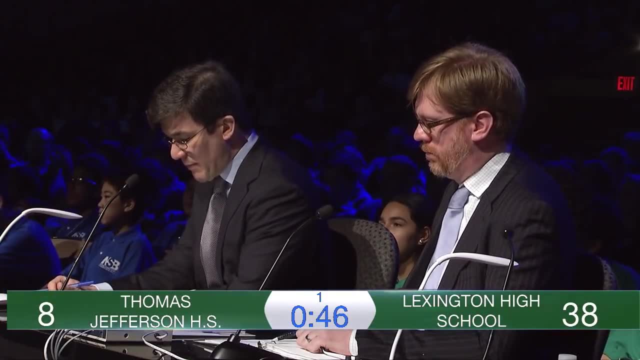 toss up earth and space multiple choice. in the late 1800s, lord kelvin estimated the age of the earth to be approximately 100 million years. by calculating how long it would take a planet of earth's size to cool from its temperature of formation, kelvin's estimation was under the true value of 4.5 billion years because he neglected what source of heat- w. solar radiation, x, radioactive decay, y, meteor impacts, z. tectonic friction, b, captain x, x is correct. your bones in earth and space is short answer. identify all the following three statements on earth's radiogenic heat flux that are true. 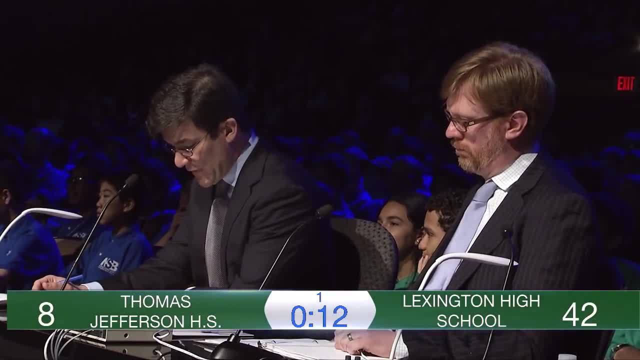 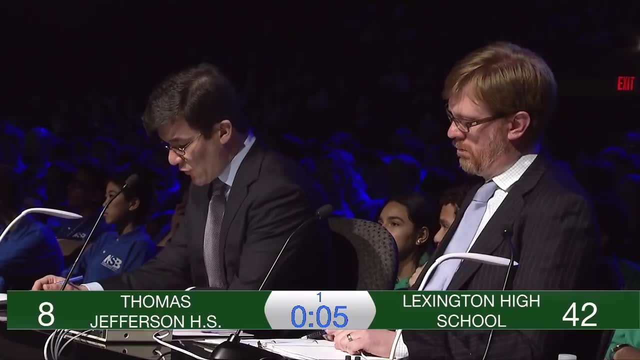 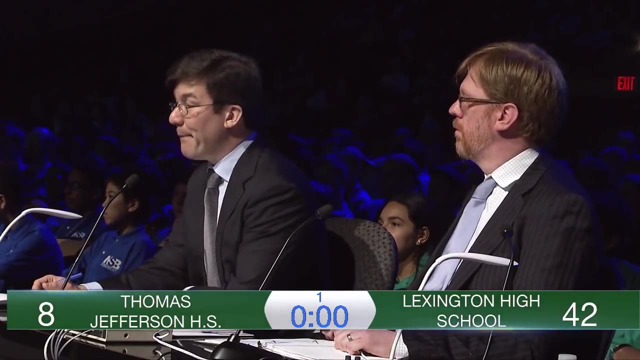 one: heat from potassium 40 decay has been relatively unchanged throughout earth's history due to its long half-life. two: uranium 235 is a greater source of radiogenic heat today than uranium 238. three: the greatest source of radiogenic heat today is thorium um half-life isn't? i mean, potassium 40's half-life isn't that long, it's like one point. 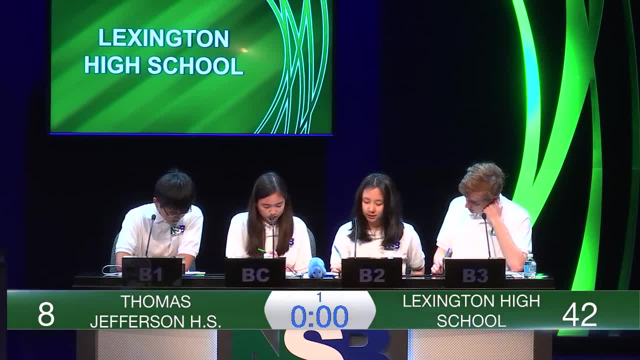 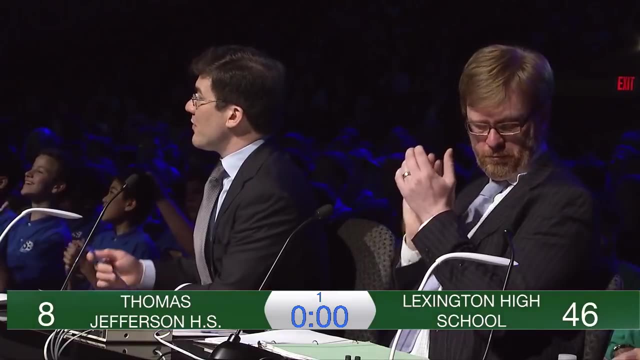 something billion years. okay, two is wrong. so i don't know if it would be, yeah, i guess what. what about number three? i don't know, maybe sure go three only. okay, three only is correct. and that is the half score at the half: lexington high school: 52, thomas jefferson eight. we'll take a two-minute break. 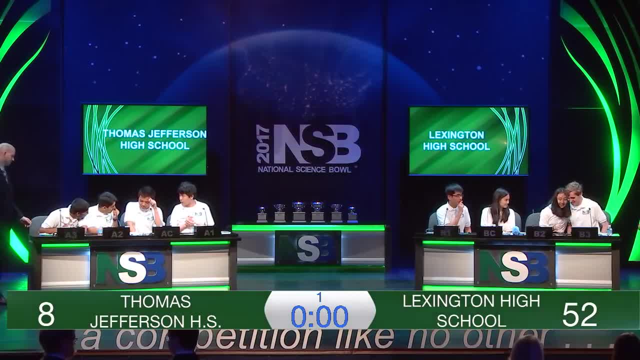 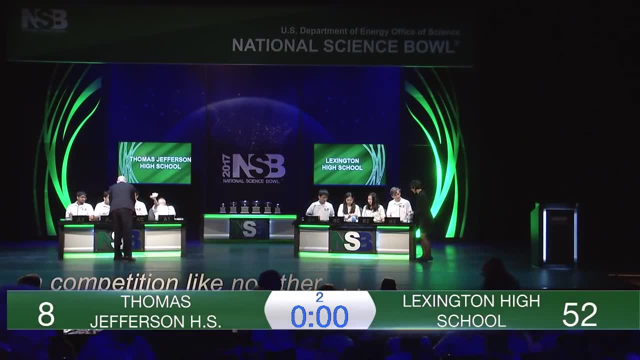 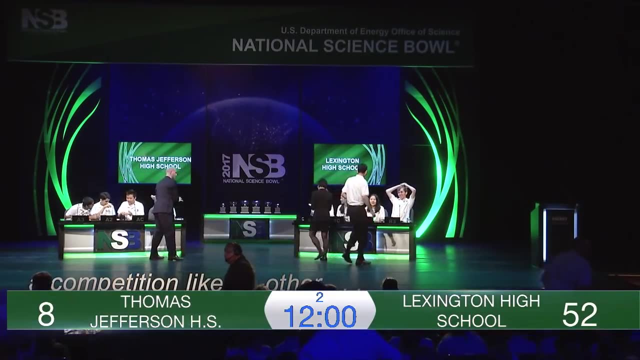 you're also like on a good, you're also like on the next one. okay, and that's a very good point. really, i think we're going to see the difference between the two, and what we're seeing now is that maybe for this one it's way too hard to rely on. but yeah, i'm not like you know, it's kind of a thing. 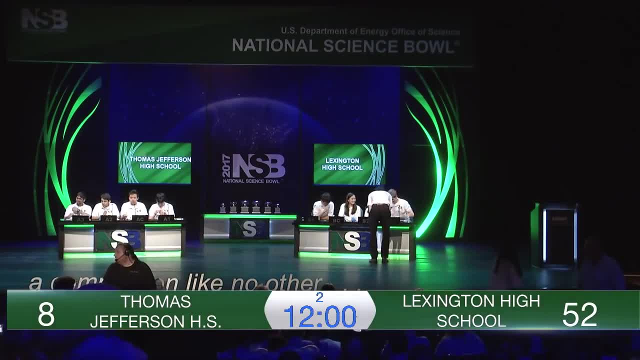 that i've experienced. i'm not like a professional, but i do think that there's a chance that it's going to be like this one. you know, after 30 years it's going to be like you know about the world and you know that there are billions of people making this thing and we're not gonna. 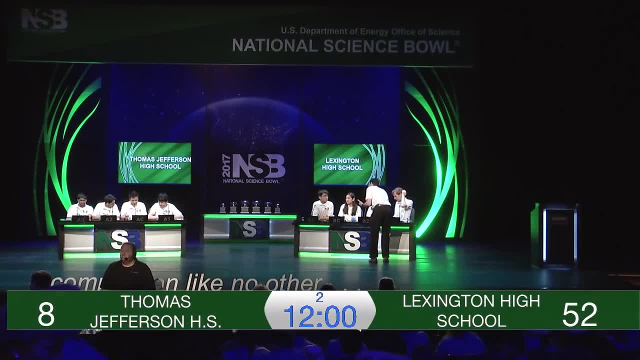 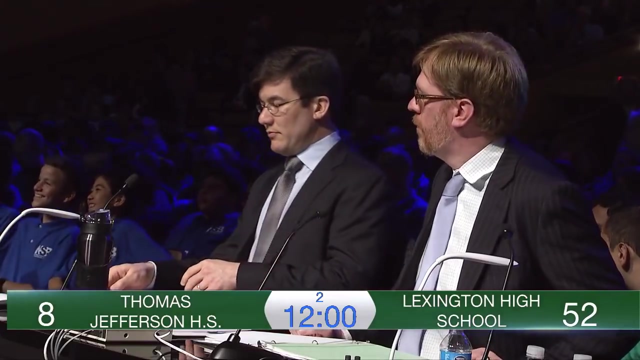 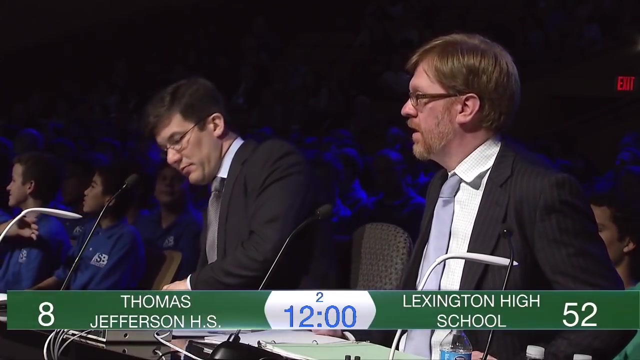 make it the same way for the rest of all of us, right? right, we're not, we're just kind of you. you please take your seats, all right? uh, just a quick reminder before we go on with the second half of uh, double elimination round eight audience. you've been fantastic and this has been uh, these rounds. 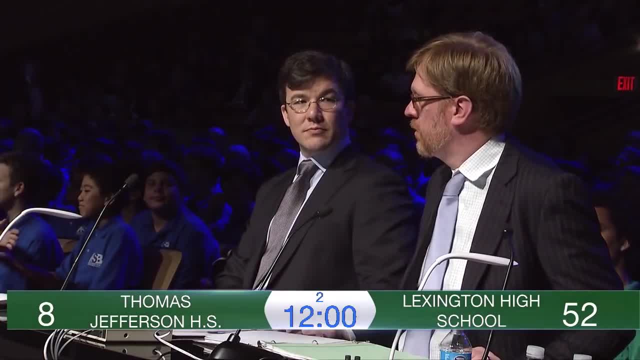 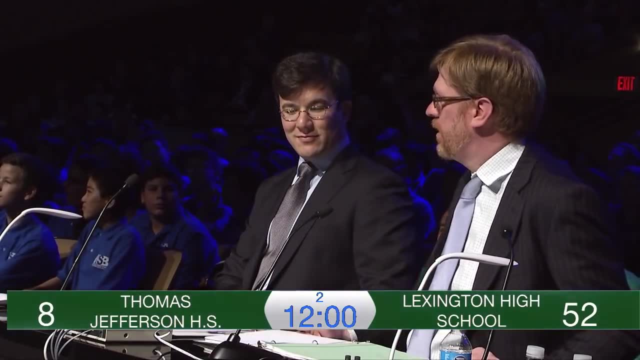 have been excellent. i just want to remind you all to uh stay silent during the round um after an answer has been given. a particularly amazing answer has been given correctly. an ooh or an ah is totally fine, but please refrain from doing it during the asking of a question. 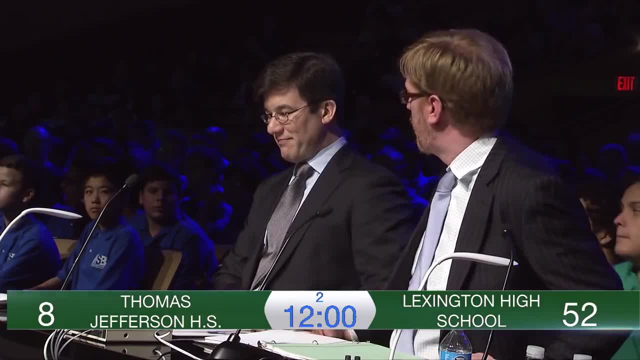 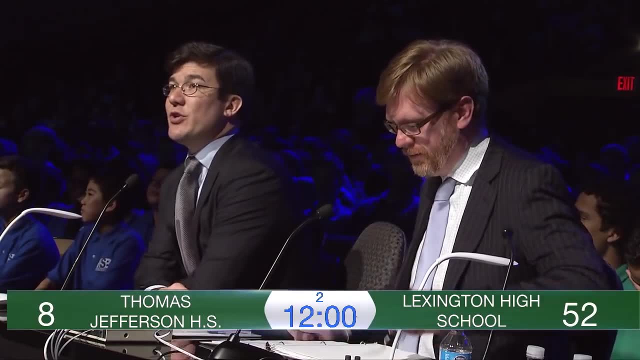 we don't want to tip our hand to any of the questions. okay, thank you very much. thank you, okay. we've gone through 12 questions in the first half. do we have any substitutions at the half for either team? okay, let's please test our buzzers again for the left side. let's. 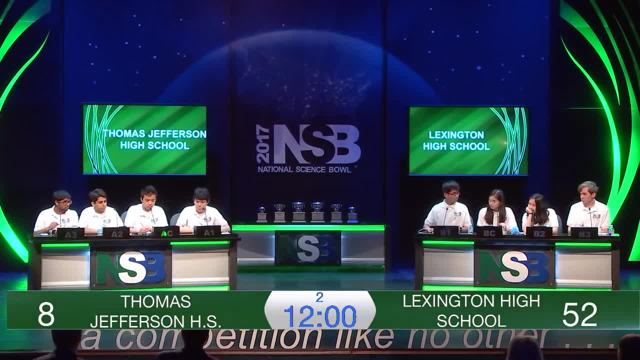 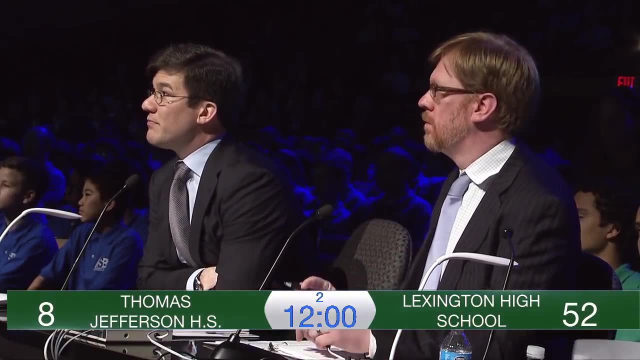 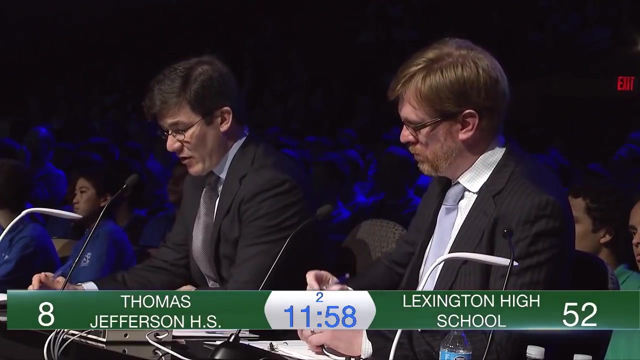 work our way across. sorry, a captain, okay, okay, thank you very much. okay, do we have any questions before we begin? are both teams ready to resume? yes, well, good luck. we'll pick up with question number 13. it's a toss-up and energy short answer. recently. department of energy researchers at pacific northwest national laboratory. 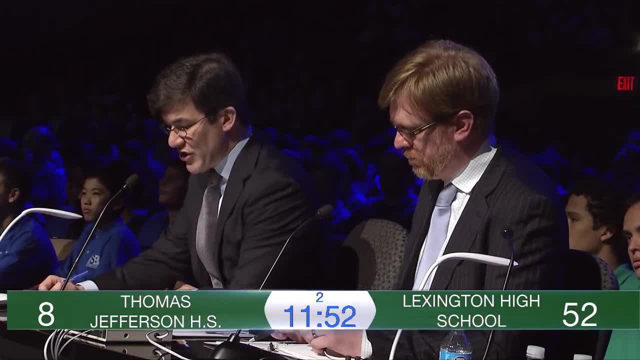 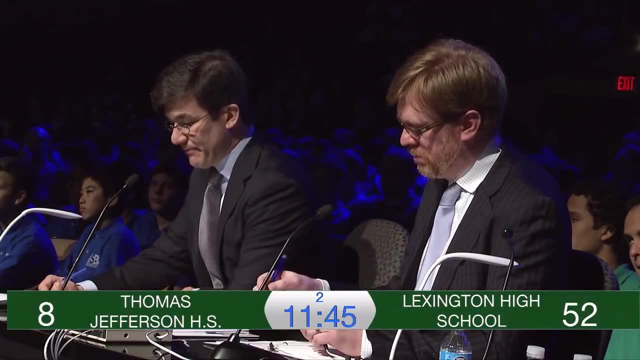 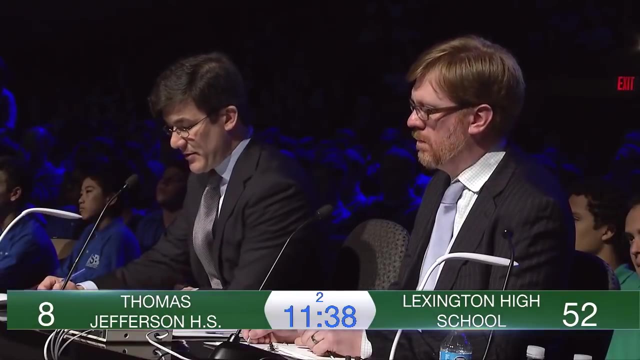 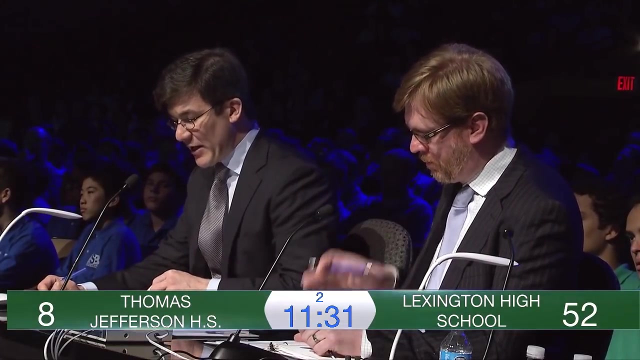 determined the last nickel catalyzed step of methane formation in methanogens. what type of spectroscopy did they use to rule out the presence of a nickel methyl radical intermediate? b1 nmr. sorry, it's incorrect. a2 icpms. no, i'm sorry, it's also incorrect. it's like it's electron paramagnetic resonance spectroscopy. 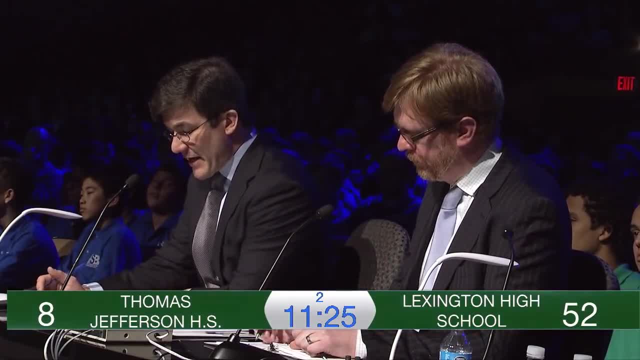 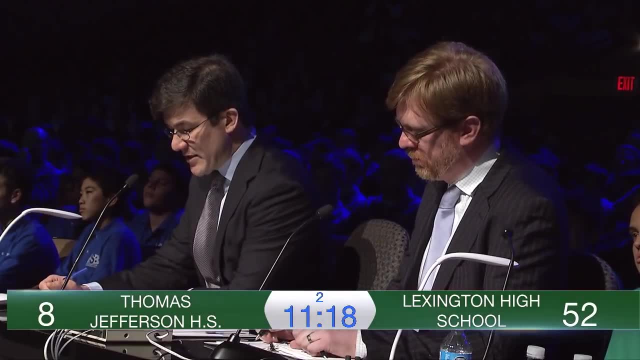 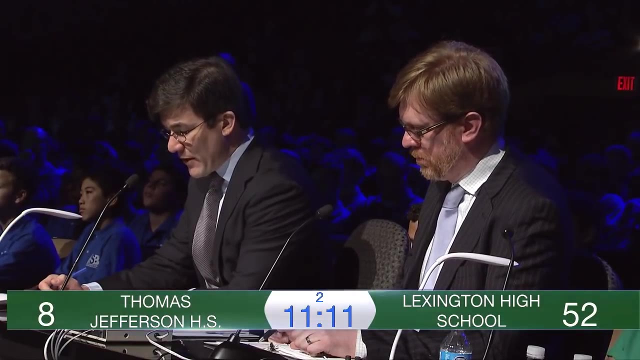 toss-up 14 is in biology. short answer: identify all of the following three statements that are true of confocal microscopy: one out of plane light is eliminated using a series of dichroicals. 2. Increasing pinhole size increases the depth of field. 3. Confocal microscopes can image up to a millimeter deep in thick untreated tissue samples. 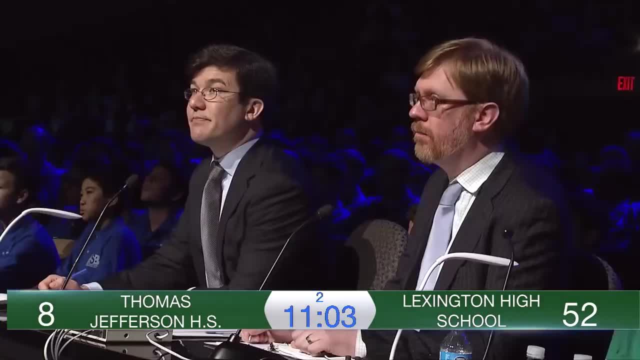 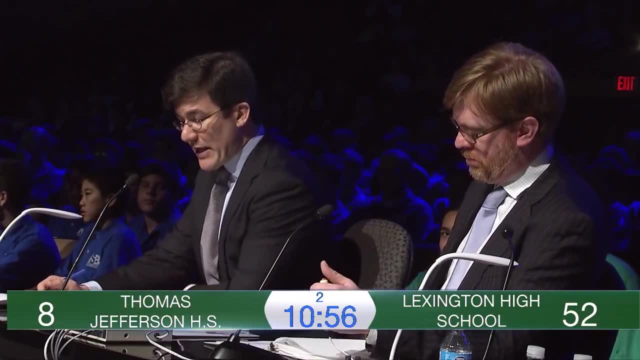 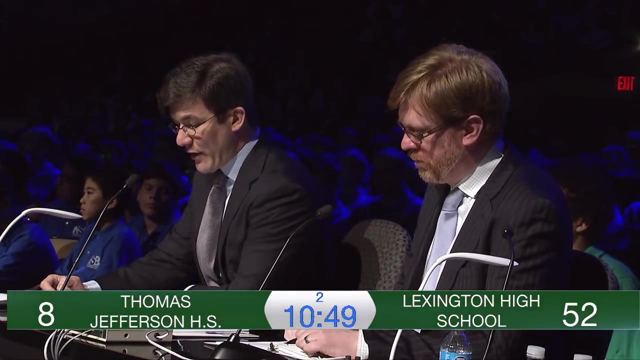 B Captain, All of them. Sorry, it's incorrect A- 3. 1 and 3 only. Sorry, it was actually 2. only Toss-up number 5 is in math Short answer: Compute the determinant of the inverse of the 2 by 2 matrix, with first row 3, 4, and second row minus 1, 5.. 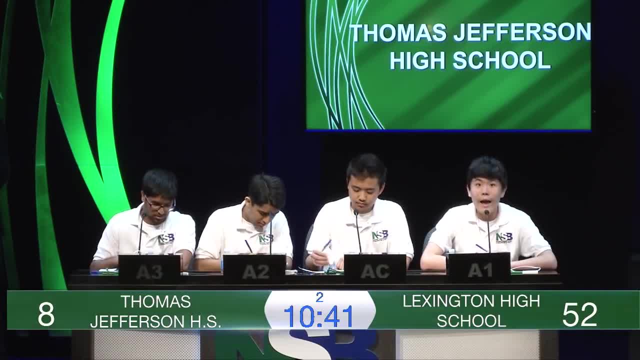 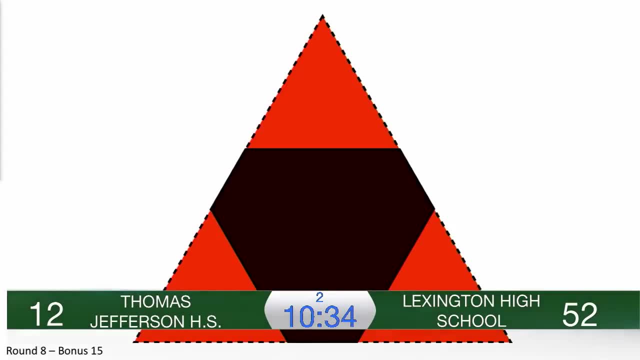 A Captain. 1, 19th Is correct. Your bonus question is visual In math. short answer: The hexagon in the center of the figure represents a top view of a sprinkler head. The sprinkler head is formed by deleting. 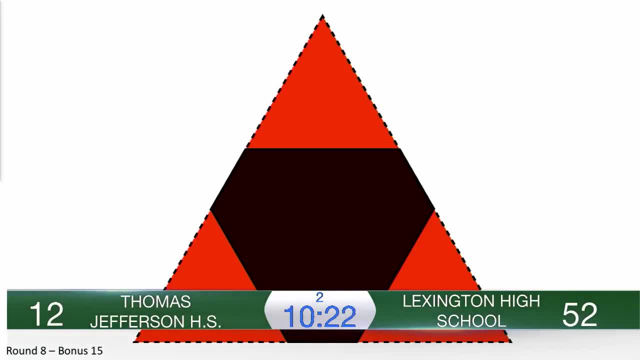 The three congruent orange equilateral triangles from a larger equilateral triangle. If the hexagonal head has half the area of the original triangle, then in the hexagon what is the ratio of the shorter side length to the longer side length? 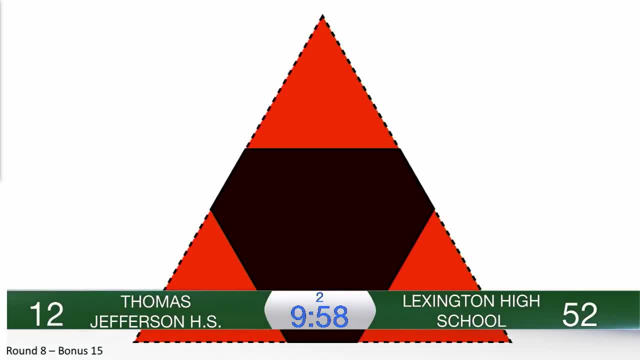 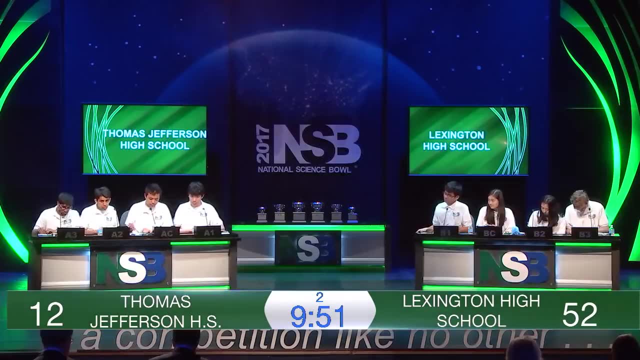 So the one is short is the longer Mm-hmm, Then we're at 6 minus 2.. I think one over is probably 6.. No, Uh, the square root of 6 minus 2. Is correct. Toss-up 16 is in earth and space. Short answer. 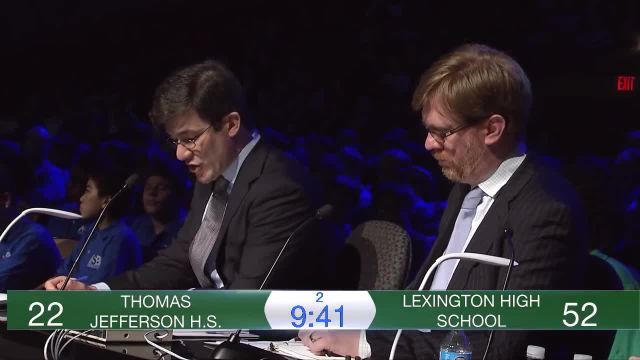 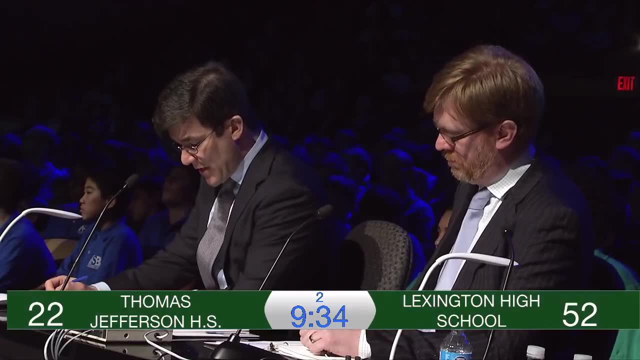 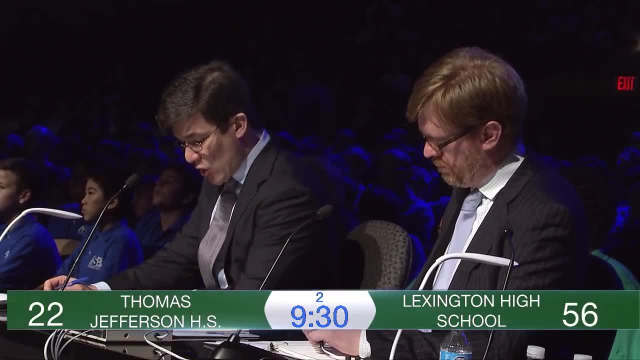 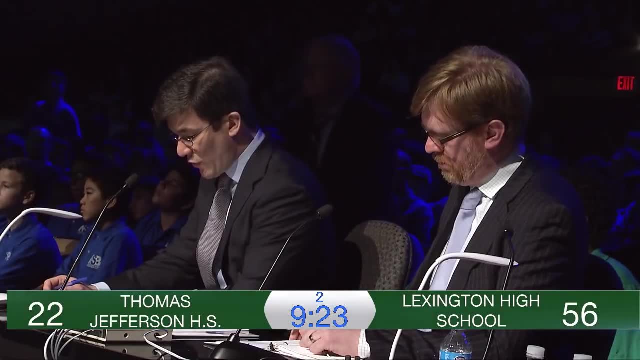 Identify all of the following four transition metals that can only be naturally synthesized in supernovae: 1, iron 1, iron 1, iron 2, gallium. 3, nickel 4, chromium 2, gallium. 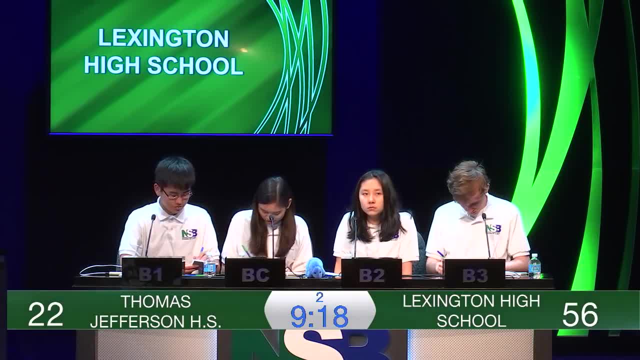 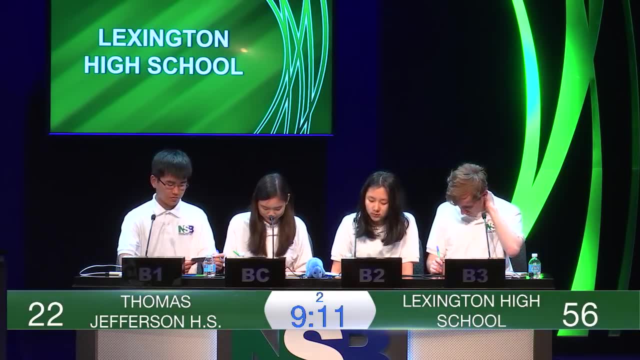 3, nickel, 4, chromium. Oh, is it everything but iron? Iron means chromium is before iron. Iron means chromium is before iron. Yeah, Oh, really Yeah, Oh, So 2 and 3 then Yeah. 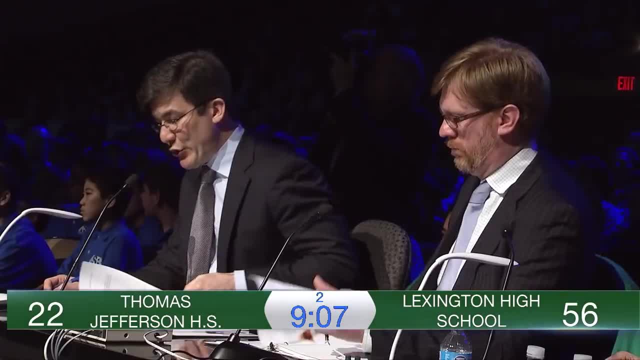 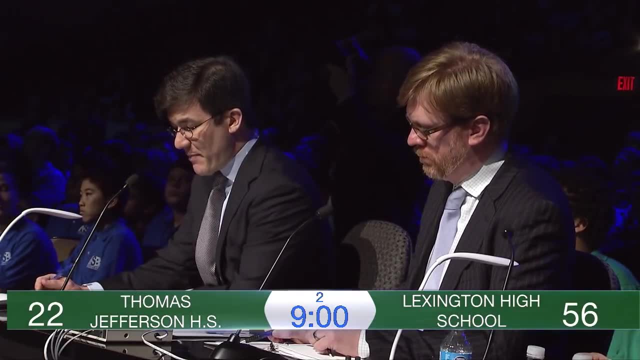 I think so. Yeah, That would make sense. Okay, 2 and 3.. Sorry, It was just 2.. Okay, Toss-up 17,. chemistry: multiple choice. Which of the following best describes the first step of a reductive amination? 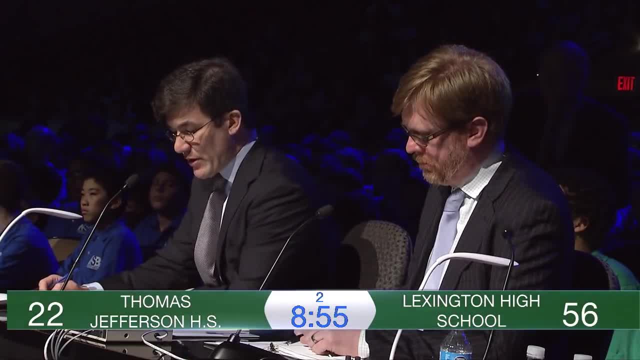 W- adding an amine to an aldehyde or carbon. W- adding an amine to an aldehyde or carbon. Toss-up 17,. chemistry multiple choice. Shown on the image is video on call or ketone Interrupt. 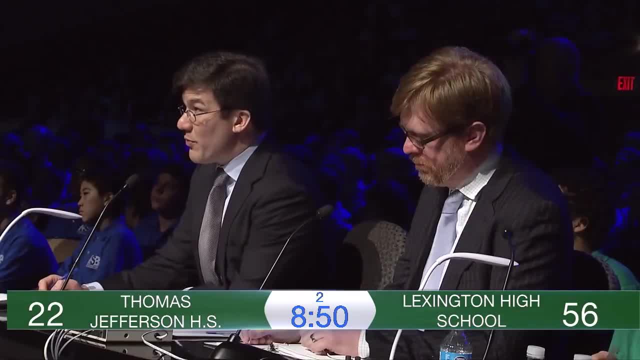 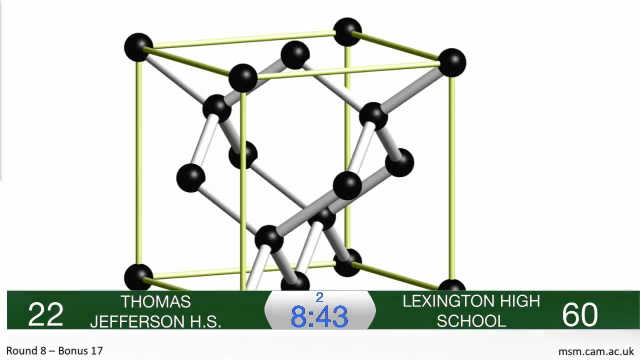 V1.. W Is correct. Good, Thank you. Your bonus question is visual In chemistry short answer. Shown on the image is one unit cell. Wait, wait, We don't see. Sorry, Chemistry short answer. 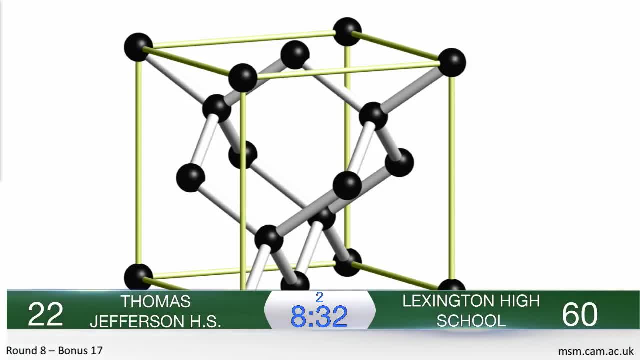 Shown on the image is one unit cell of a diamond cubic crystal structure where black spheres represent carbon atoms. Answer the following two questions: 1. How many carbon atoms are in each unit cell? 2. Is the packing efficiency of this lattice higher, lower or equal to that of an FCC lattice? 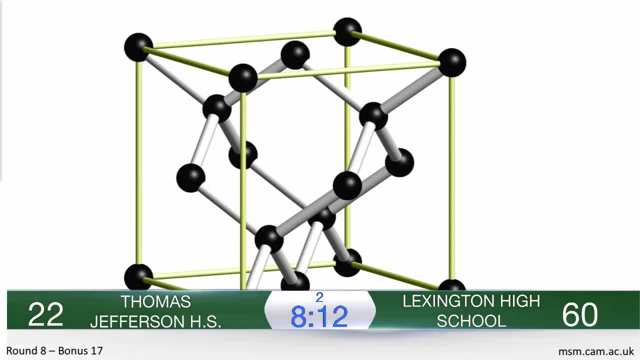 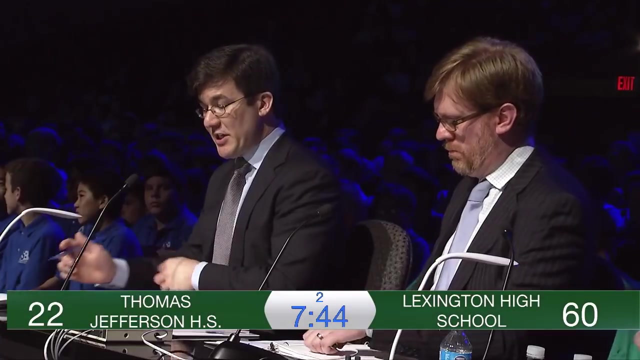 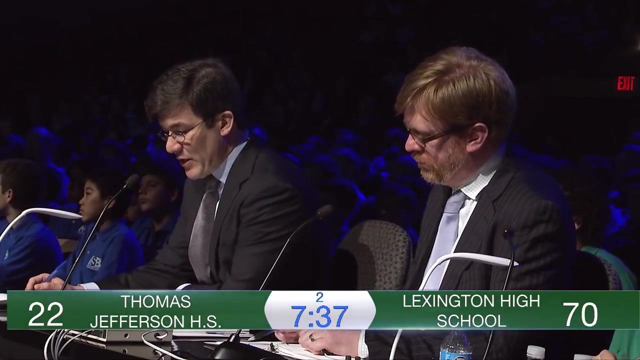 1 is 8,, 2 is lower. That is correct. Toss-up 18 is for both teams in physics. Short answer: The action of the system is defined as the time integral of what quantity, which equals the difference between kinetic and interrupt. 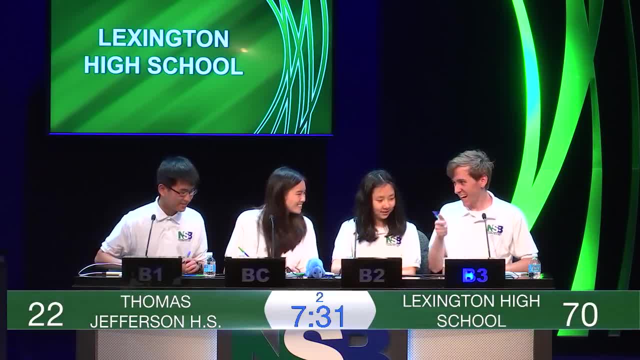 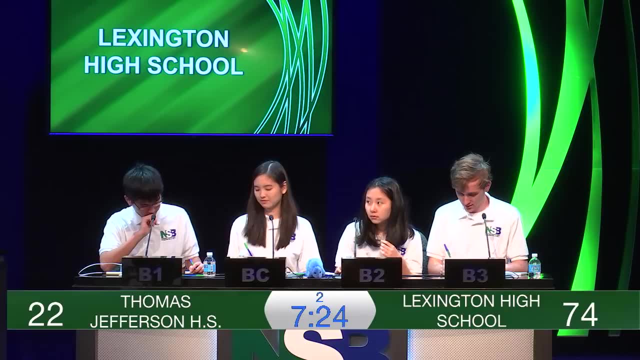 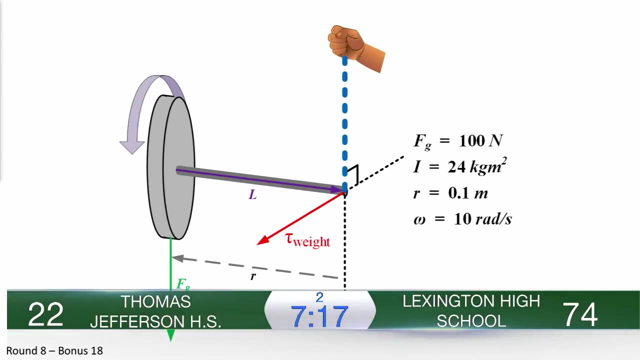 B3.. Lagrangian Is correct. Your bonus is visual in physics and it is short answer. Shown in the image is a spinning bicycle wheel that is suspended by a blue string from its axis, Which is 0.1 meters long. 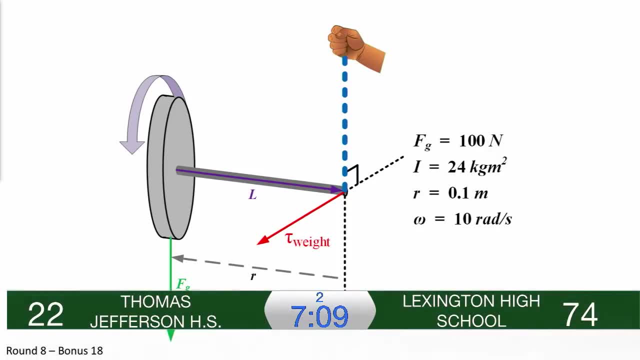 A relevant force body diagram is shown and the moment of inertia, angular speed and weight due to gravity of the wheel are also given In seconds and in terms of pi. what is the period of precession Seconds under pi 37?? 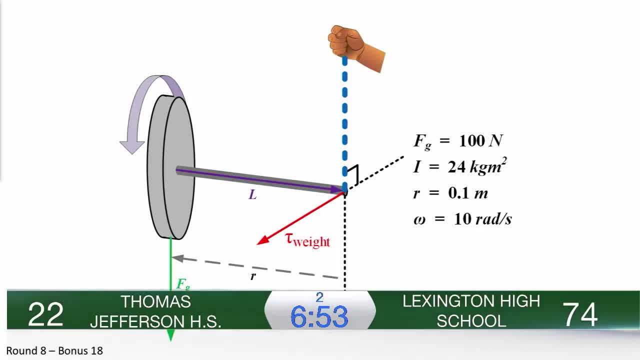 Yes, It would be 1 over that right. Um, All right, There you go Over M or G, Since this one is seconds away. Okay, I would Come on. We should really guess this. I don't know. 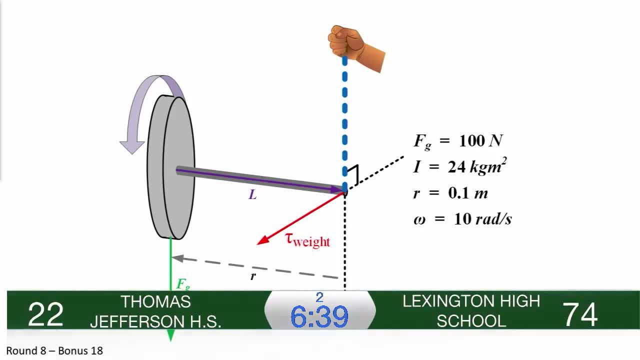 No, we haven't. So 10. 20 pi, I'm gonna go with 20.. Five seconds: 1 over 24. 24 pi. Sorry, it's actually 48 pi. Toss-up 19 is in chemistry multiple choice. 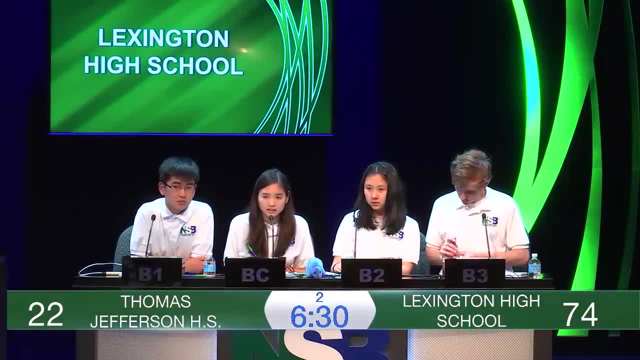 Which of the following statements is the best explanation of why silver fluoride is soluble in water? W. Silver I is a hard acid and fluoride is a liquid. What is the best explanation of why silver fluoride is soluble in water? W. Silver I is a hard acid and fluoride is a liquid. 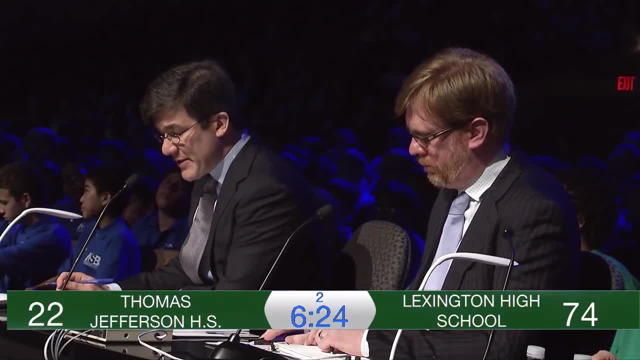 Toss-up 19 is for both teams in physics. Short answer: Which of the following statements is the best explanation of why silver fluoride is soluble in water? W- Silver I is a hard acid and fluoride is a hard base. X- Silver I is a soft acid and fluoride is a hard base. Interrupt B1.. X Is correct. Thank you. Your bonus question in chemistry is short answer. Identify all of the following three protecting groups that are labile at pH 1 but stable at pH 12.. 1. Dimethyl acetal. 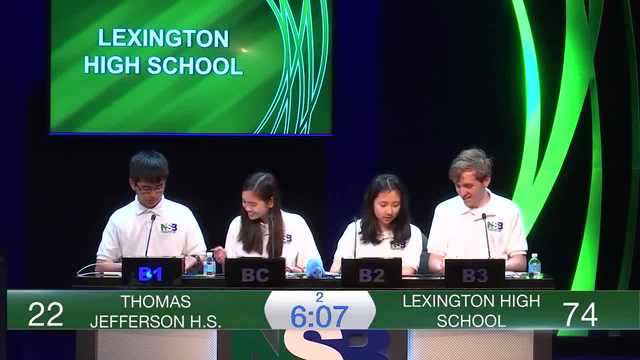 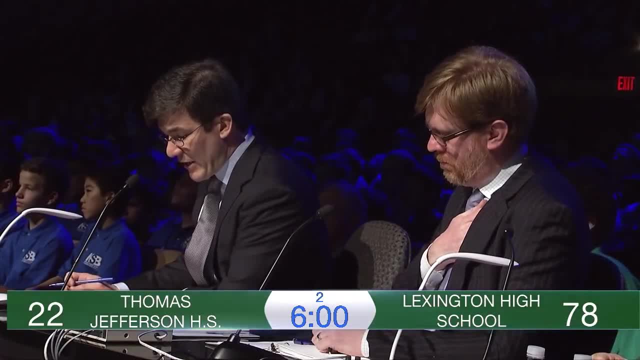 2. Methyl ester. 3. Chlorine, 4. Chlorine, 5. Chlorine, 6. Chlorine, 7. Chlorine, 8. Chlorine, 9. Chlorine, 10.. 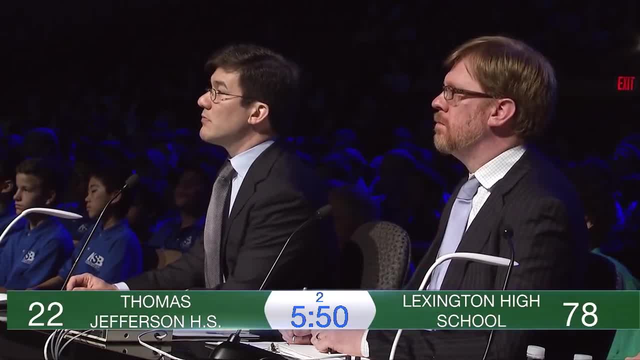 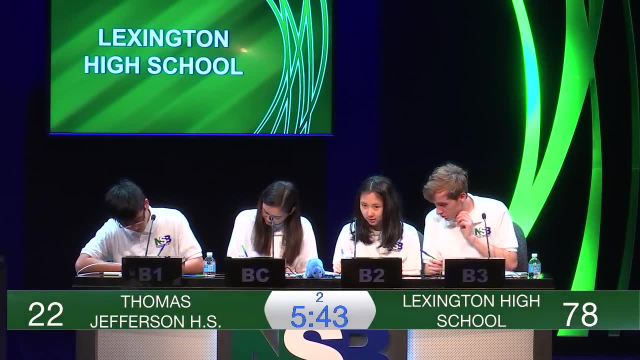 Chlorine Undercurrent: 10. Chlorine, 11. Chlorine, 12. Chlorine, 13. Chlorine, 14. 3. 3. Bach protected amine. What was the first one, Acetal? 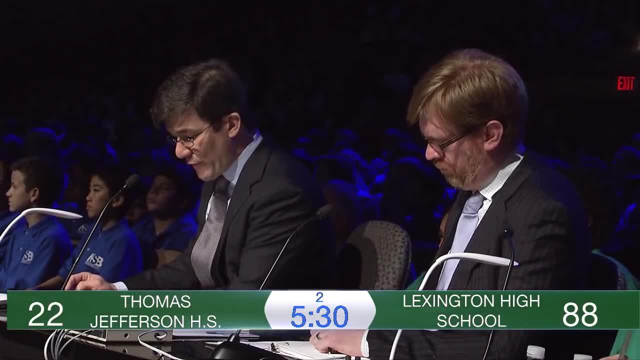 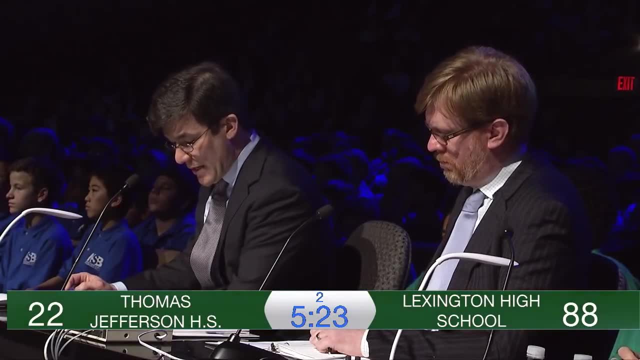 OK, 1. And 3. Is correct Toss up 20s in physics, Multiple choice. Which of the following statements is true about steady laminar flow between two stationary parallel plates: W, X. the velocity profile is parabolic. about the center line. 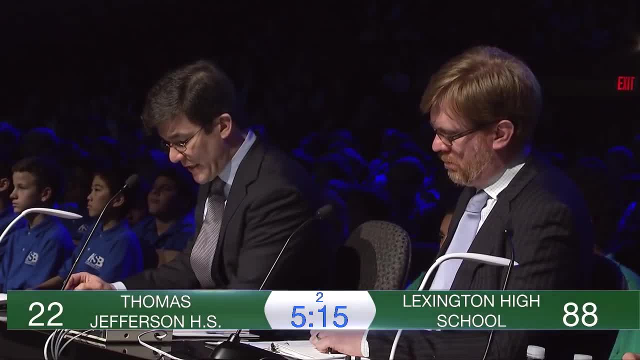 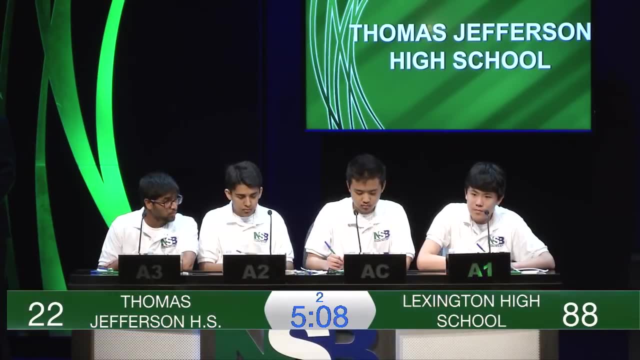 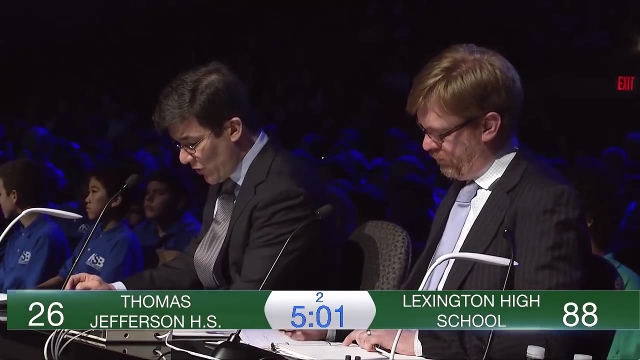 Y: the velocity profile is linear and increases towards the top plate. Z: the velocity profile is not dependent on the pressure gradient A1.. X Is correct. Your bonus in physics is short answer. Bob observes Alice moving at half the speed of light towards his left. 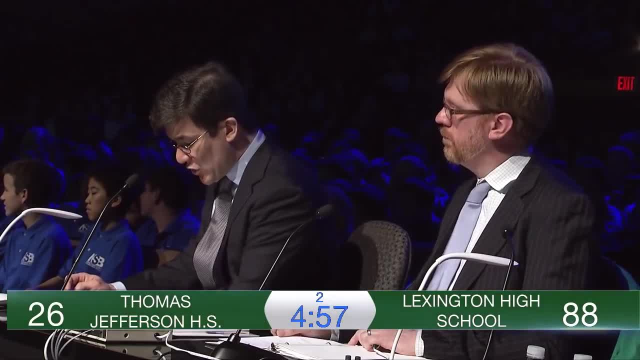 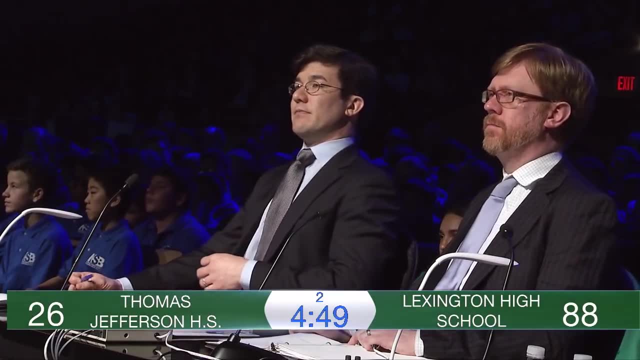 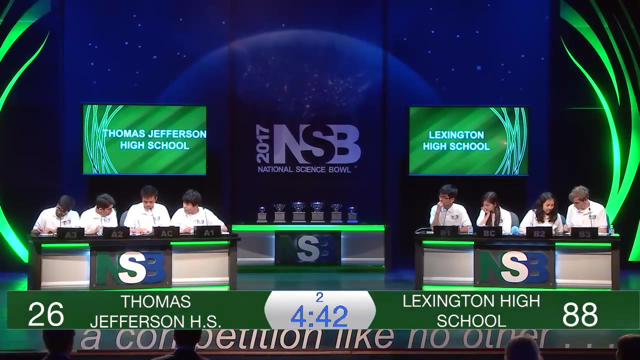 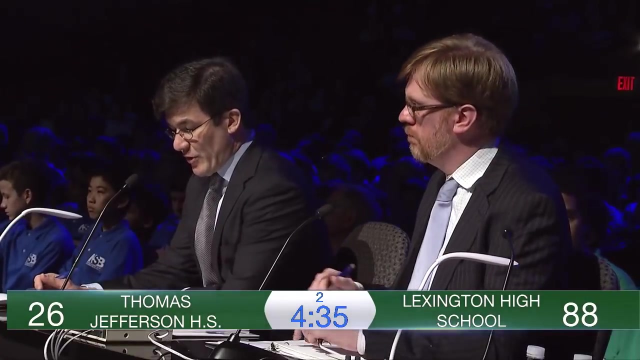 and Carol moving at half the speed of light towards his right To the nearest 10,. Alice will measure Carol's speed to be what percentage of the speed of light? 80. Is correct. Toss-up 21,: energy short answer. 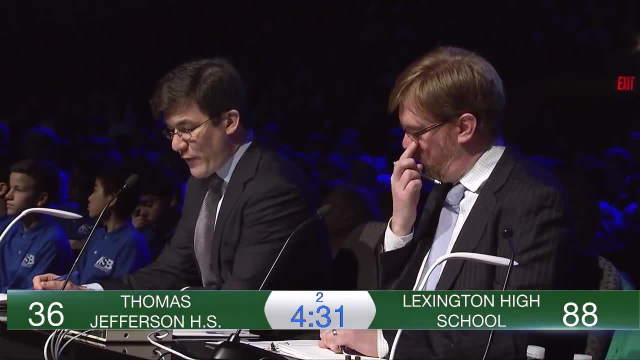 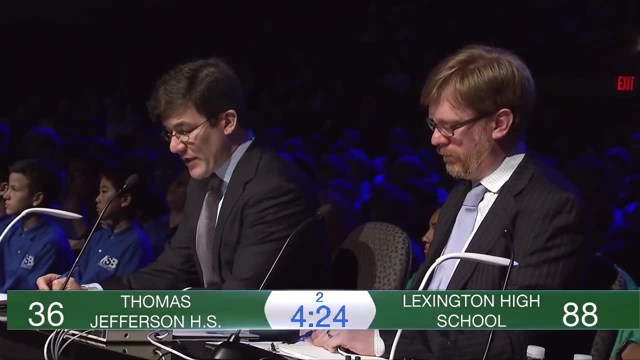 Researchers at the Department of Energy's Advanced Light Source measured photoionization cross-sections for C60 fullerenes and detected that the energy of the light source was not as high as the speed of light. They detected a surface mode where all 240 electrons in the buckyball were collectively excited. 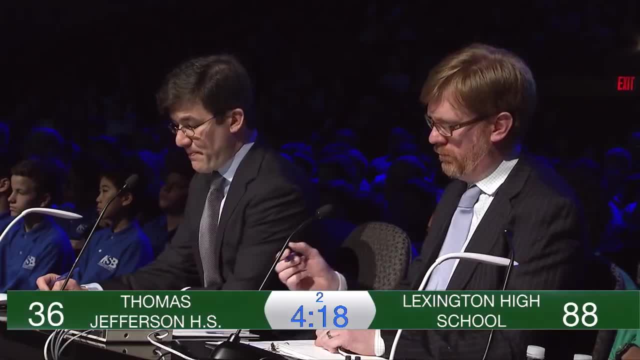 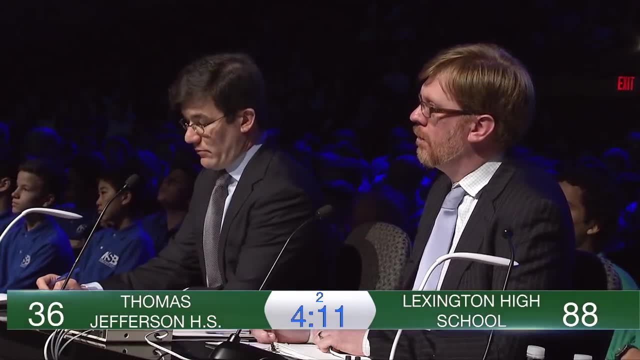 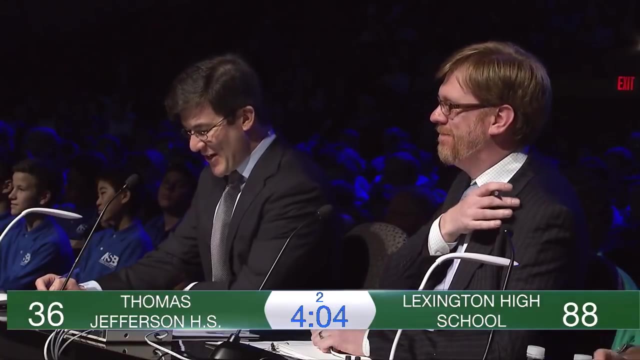 What term is given to describe a collective motion of this type? A1. Resonance- I'm sorry that's incorrect. B captain Flash mob. Sorry, no, it's actually called a plasmon. Toss-up: 22, biology- short answer. 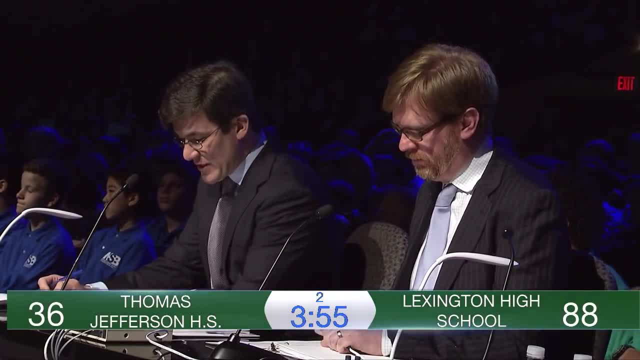 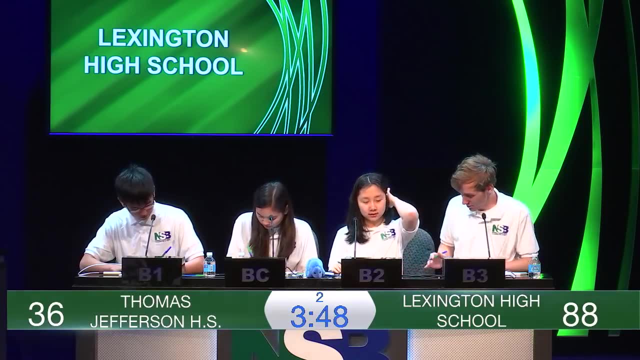 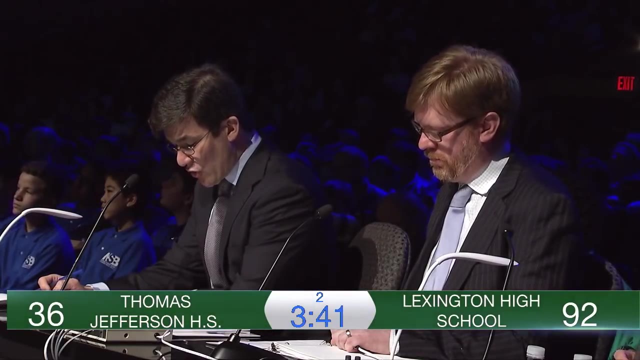 Connections are transmembrane particles, proteins that compose. what type of intercellular junction B captain Gap junctions Is correct? Your bonus in biology is short answer. Rank the following three biological structures in increasing order of cholesterol concentration in their outer membranes: 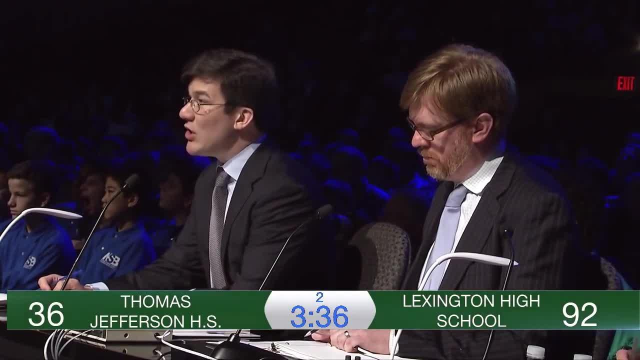 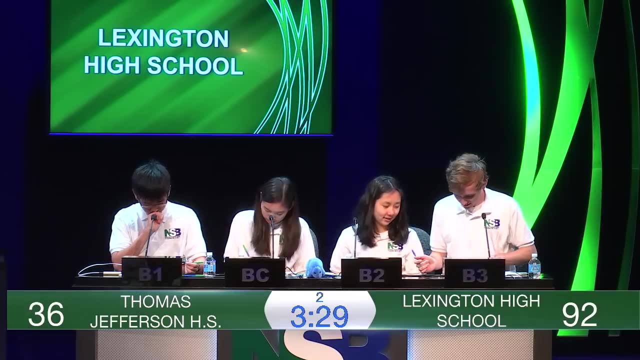 One red blood cell, Two E coli, Three mitochondrion Increasing, so it's probably two, three, one Good Mitochondria. Well yeah, they're like weird- 54. Yeah, okay. 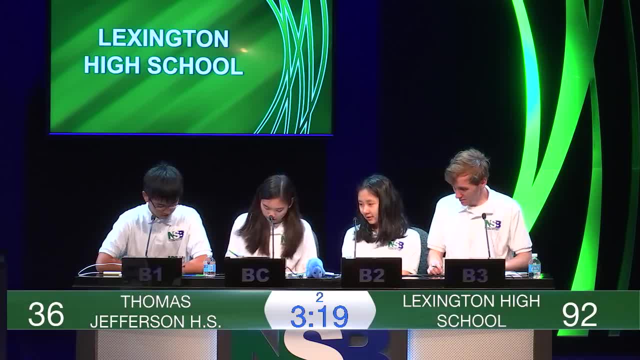 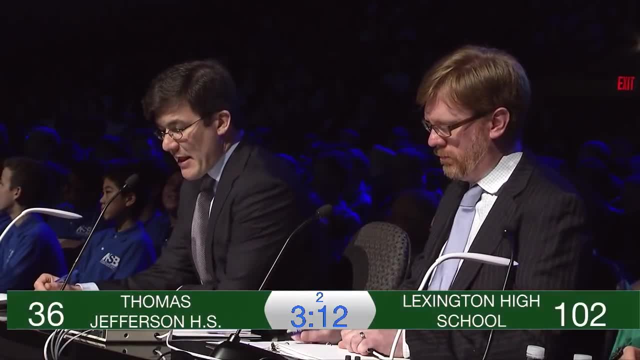 So we're not in here. Anything we do doesn't matter. Five seconds, Oh okay. Two, three, one Is correct. Toss-up 23 is for both teams in math and it is short answer. Let f of x equal the greatest integer, less than or equal to x. 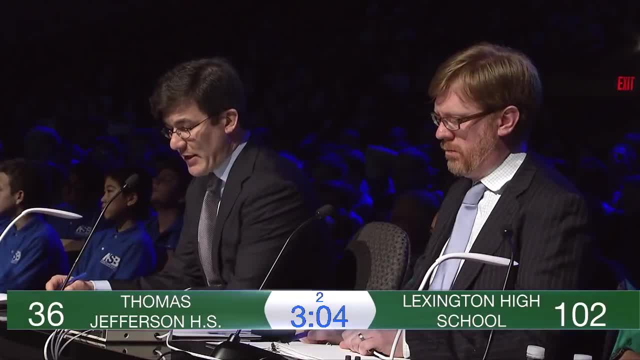 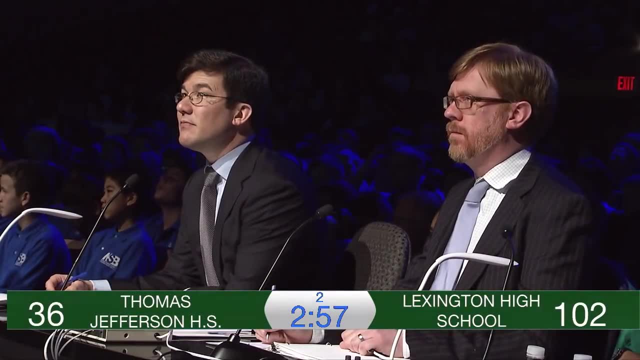 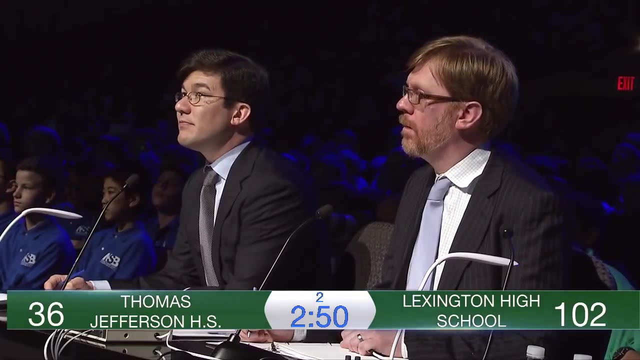 If f of open parentheses 0.2x close parentheses equals minus 25,, what is the largest possible integer value of x A captain Negative 54.. I'm sorry that's incorrect. B 2. Minus 129. Sorry, it's minus 121.. Toss-up 24 is an earth and space short answer To the closest integer. what is the ratio of the energy radiated by 7.8 earthquake to that radiated by a six-point interrupt?